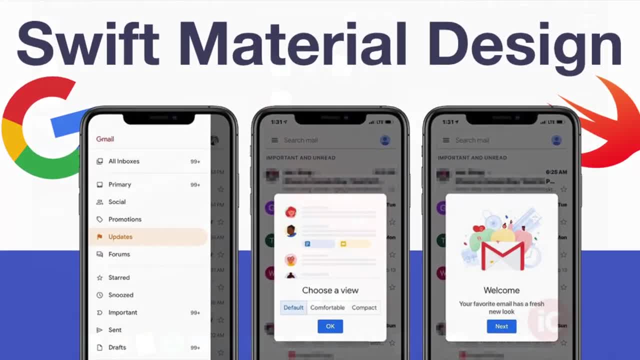 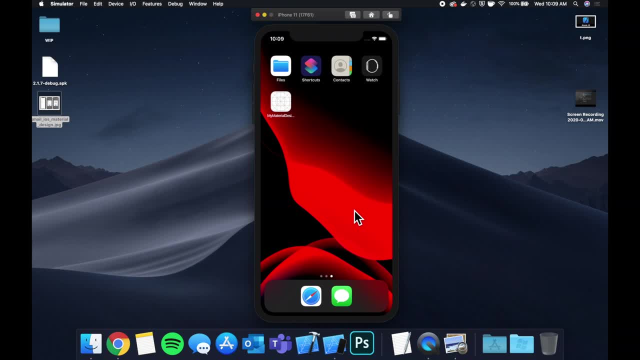 What is going on, guys? Welcome back to another Swift video. In today's video, we're going to be looking at how you can use Google's components- the ones that they use in their apps, like YouTube and Gmail- in your apps. So, specifically, their design, language and their components are called. 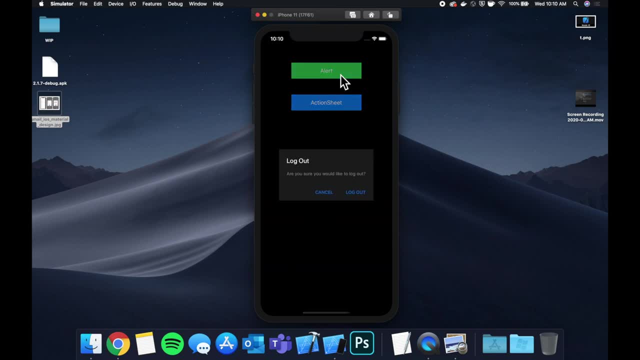 material design. And if we go ahead and hit this button here, you'll see that this alert looks a lot like the alert that you see in the YouTube app or in the Gmail app, And you can see it's also fully dark mode supported. We're in dark mode right now, And same thing for this action. 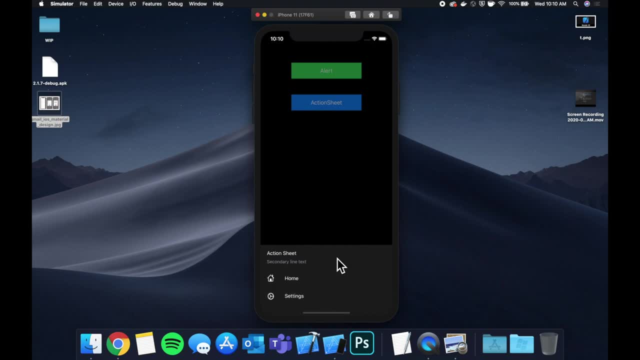 sheet, not the Apple standard one, it is the Google one And you can actually swipe it up and down to when you get all of this functionality- the icons, title, subtitle, all this stuff out of the box. So, basically, we're going to look at how to put our apps together to look like Google's. 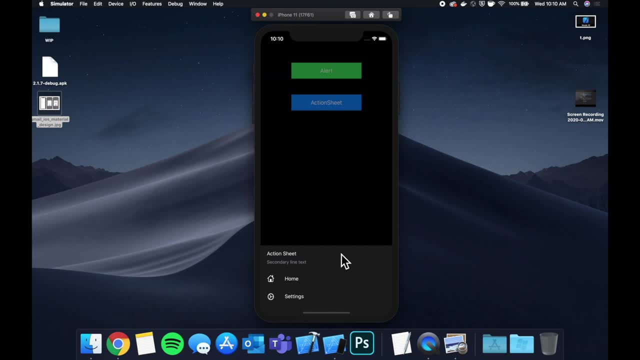 apps with really polished components, using their materials. So, that said, if you haven't smashed that like button already while I was blabbering on the beginning of this video, make sure to do so for that YouTube algorithm. Get Xcode ready, get. 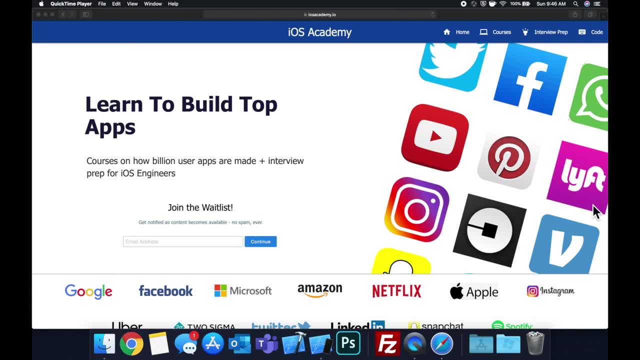 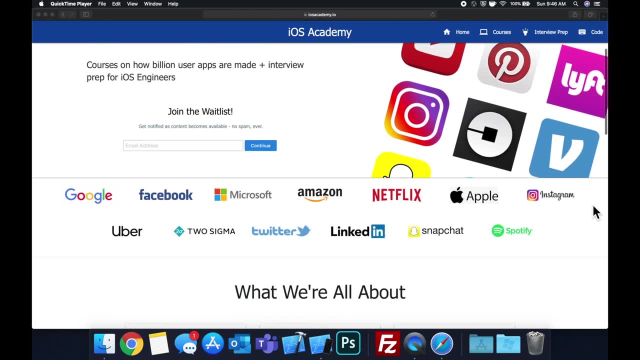 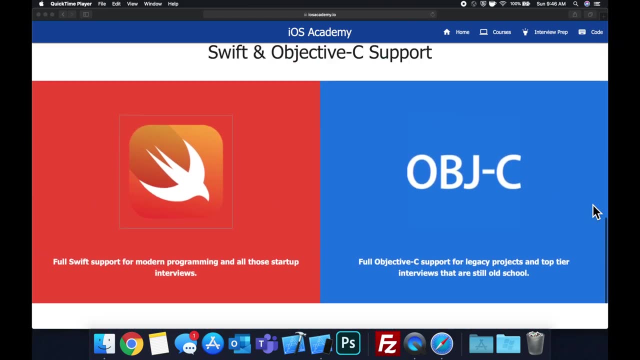 excited and let's jump right in. Quick pause before we get into the video, If you haven't seen it already. I am hard at work putting together iosacademyio, a community where all of us iOS engineers can come together, learn how to build some of the top apps like Google, and then we can. 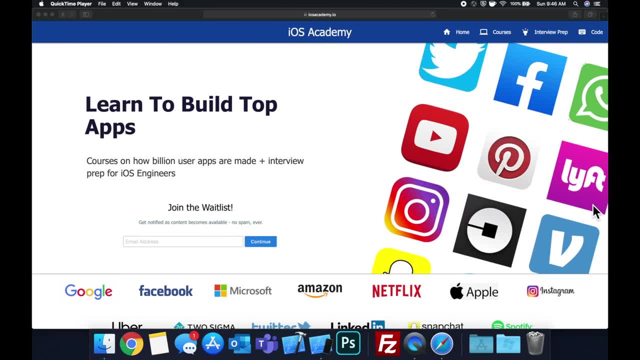 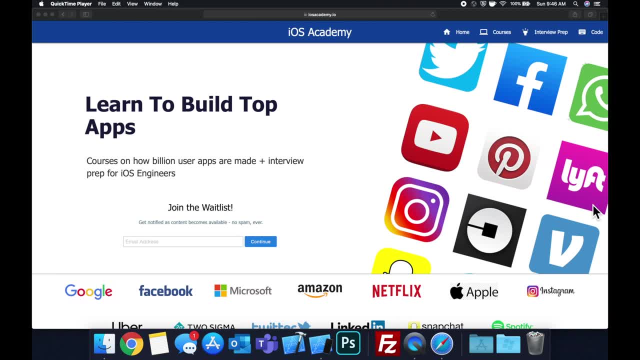 at top tech companies. So if you're interested in the free and premium content to come head on over to iosacademyio and enter your email address in the waitlist form and you will be notified as content becomes available. That said, let's get into the video, All right, so let's jump right in. 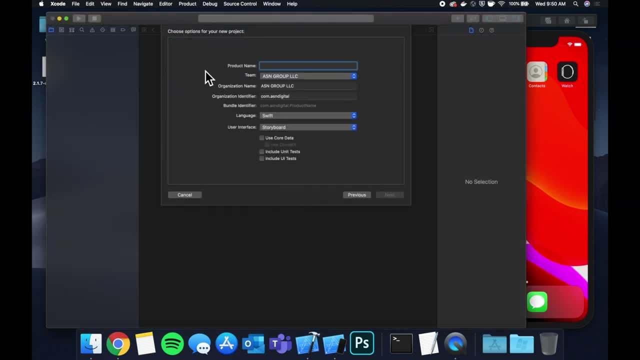 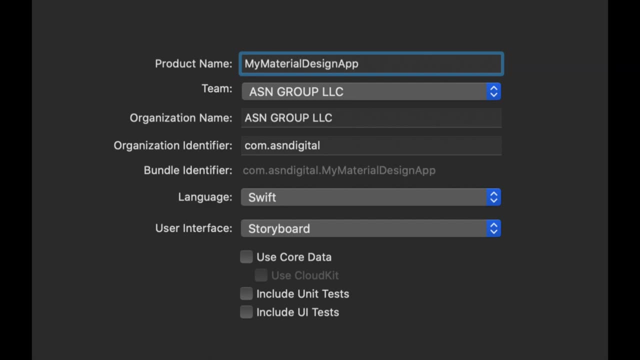 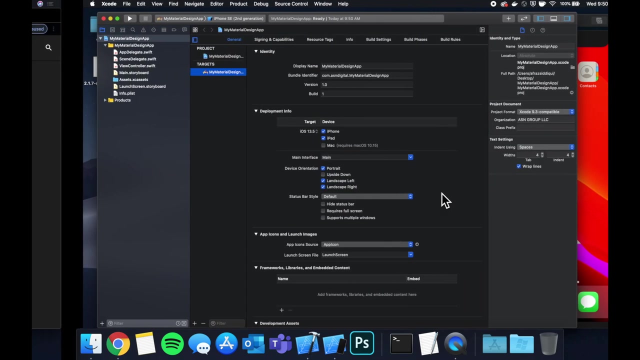 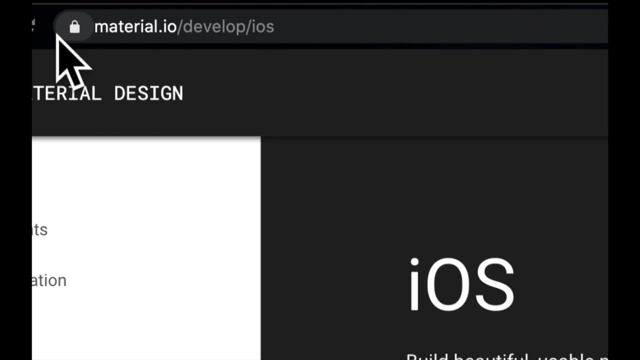 we're going to stick with a single view application template And let's call this project my material design app, And I'm going to save it to my desktop, And the very first thing we want to do is actually head on over to our browser and go to this website, which is materialio slash develop. 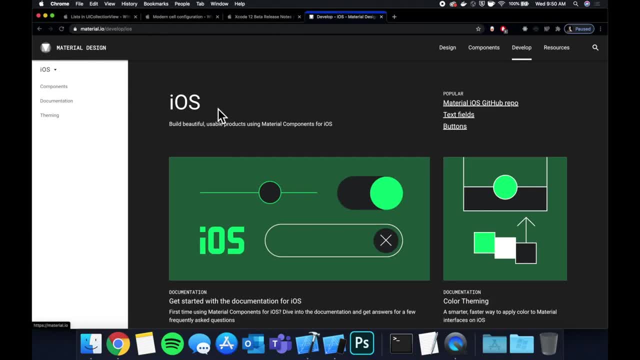 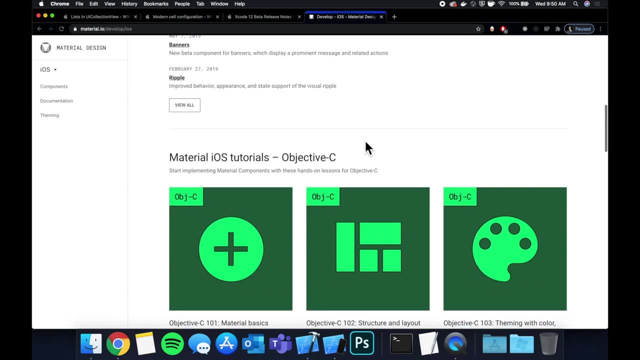 slash iOS. So, like I briefly mentioned at the beginning of this video material, design is a design language at Google that they've kind of perfected over several years And they've created all these libraries for iOS Android websites where there's a collection of 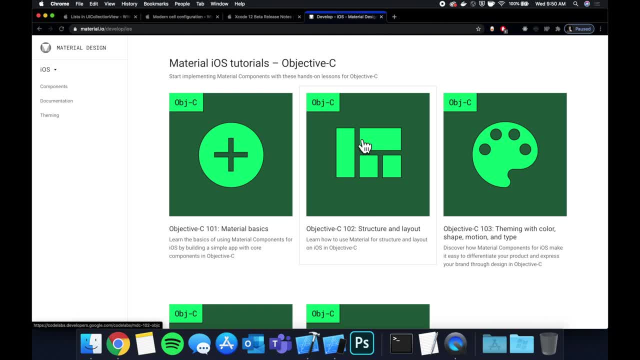 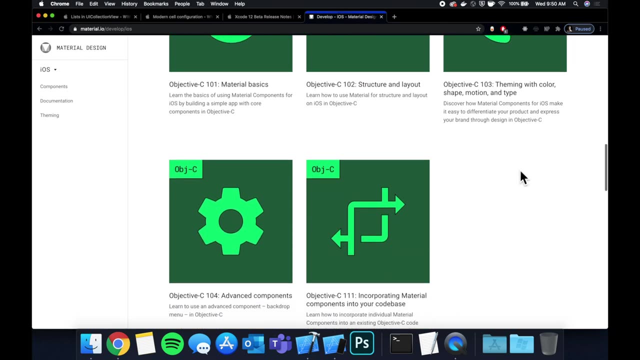 components that are consistent to their design guidelines. They've invested a lot of work in making sure is everything is accessible. dark mode supportive works in landscape, iPad, iPhone And, of course, Google uses this library and these principles and all of their 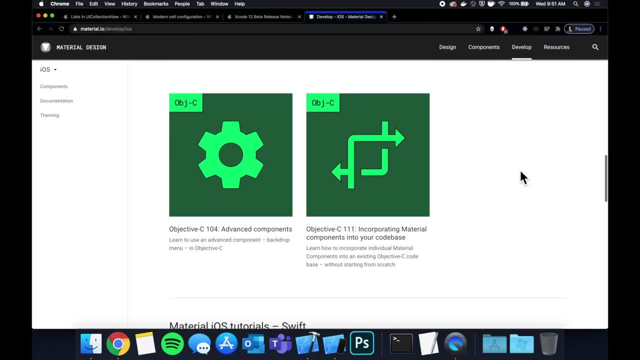 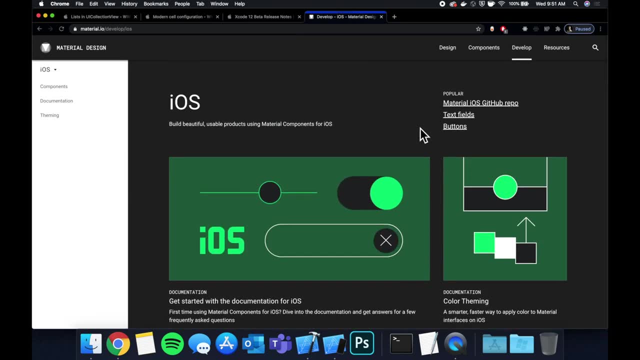 apps. So if you've ever used the YouTube app on iOS, or any of the Android apps or any of Google's websites- Google Search, Gmail- which you know I'm sure every single person watching this video has- you have seen these components. So we're going to demo two of the components, But let's 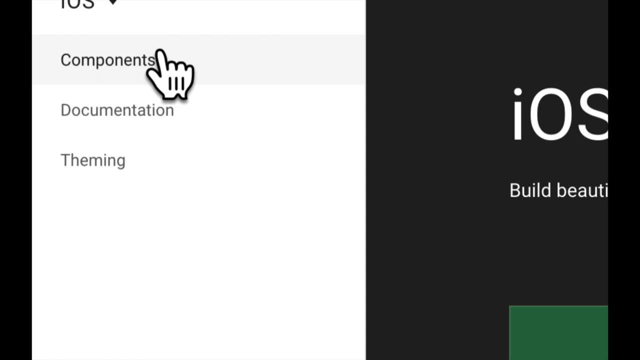 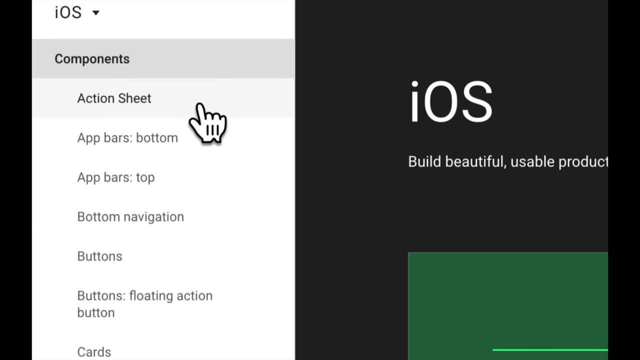 actually go through a few of them just to look at the docs So you guys can see what's available to you. So if you open up components over here, you can see there's an alphabetical list of all the things that are available. There's things like: 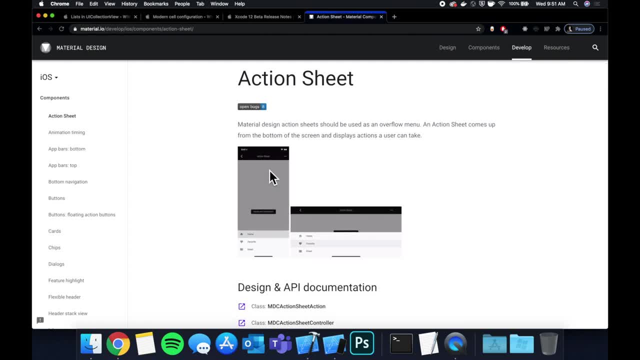 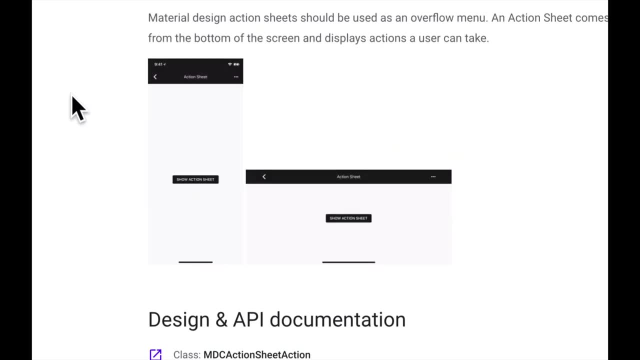 action sheet. if we click on this, you'll see a preview, both portrait and landscape, And this is the same action sheet you'll find in, like the Gmail app or the YouTube app. What else is cool in here? I really like the way. 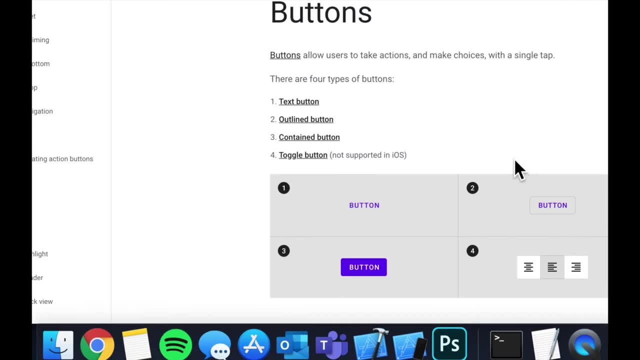 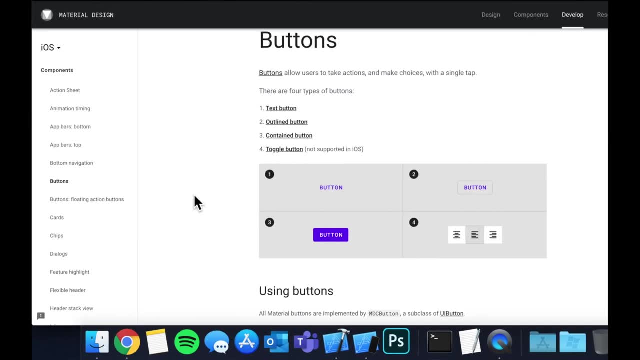 their buttons look. They're pretty standard buttons but they're polished with their borders and shadows And you get a variety of kind of looks and feels for icons or with text. I'm also a big fan of cards, if I can find them. 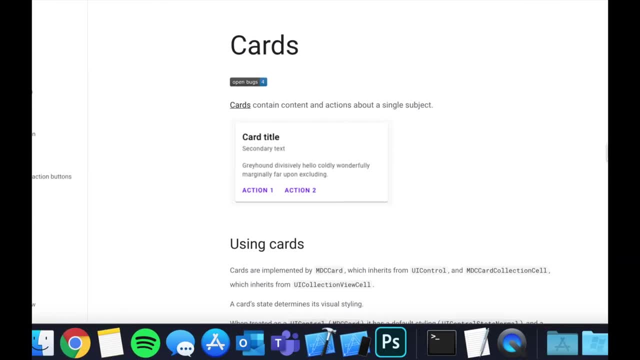 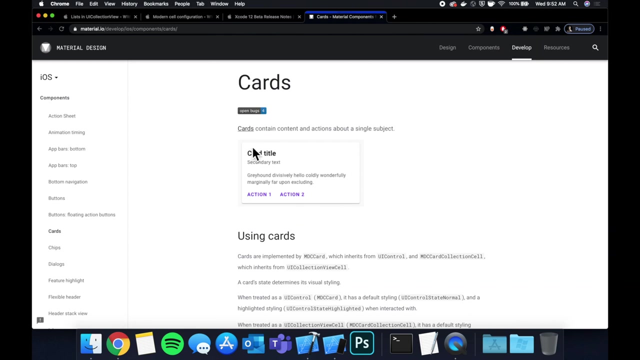 So Google uses these cards all over the place. I think this is how Google search results look today, unless they've updated it again- where you have your title, a subtitle, some content and then some action buttons and you have a really nice container. Now, under the hood, this is all just a UI view and you can build it all yourself, But obviously using a library speeds up your development quite a bit and it makes sure that everything is very tested, bug free and consistent. 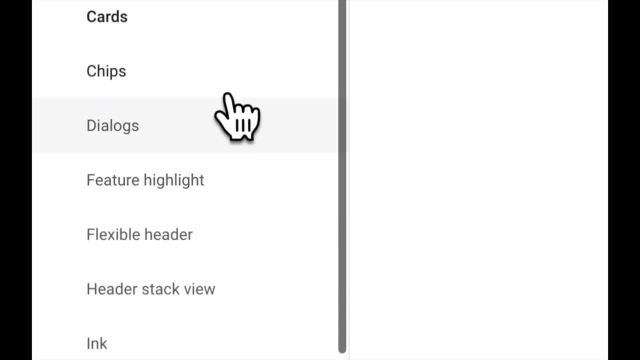 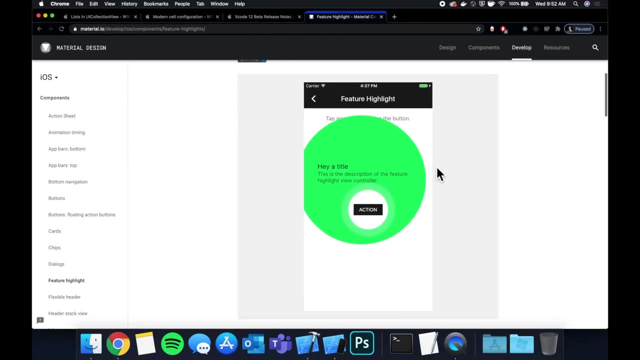 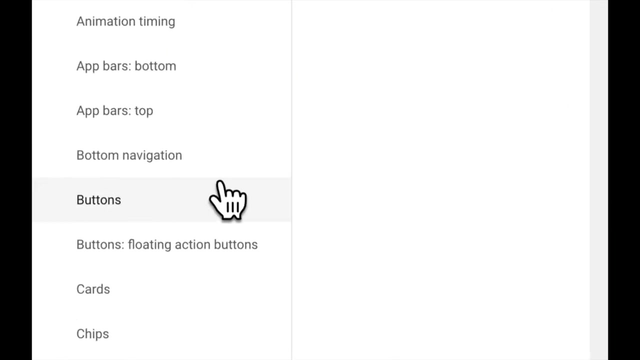 Let's see what else is cool in here. So there's cards, chips, dialogues. feature highlights are pretty nifty, So you've probably seen this on websites. Whenever Google launches something new, they'll, you know, do this little circular thing where it kind of highlights the actual feature with a description. But anyways, let's actually look at- we're gonna be looking at- action sheets and dialogues, since they're the most common components that people like to use and they're all over the place in apps. So you can see these cards, chips, dialogues are basically this thing, And you're almost- I'm almost- positive- every one of you have seen this in the YouTube app or Gmail. So let's get started over here and execute by actually closing the project with a command W, And we're going to want to open a terminal And we're going to CD into our project And we're going to bring all of these things in via Cocoa Pod. So you're going to do a pod in it And then, once that returns to an open pod file and you're able to read your project, And then you're going to click on the 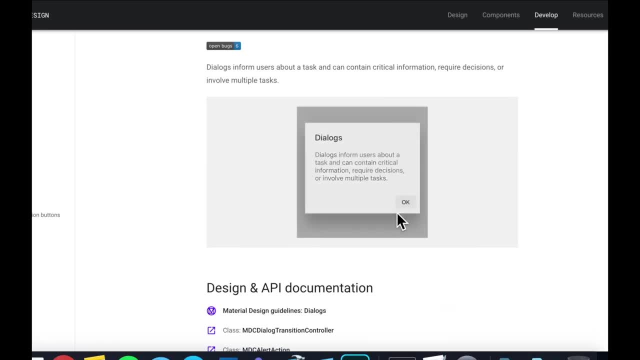 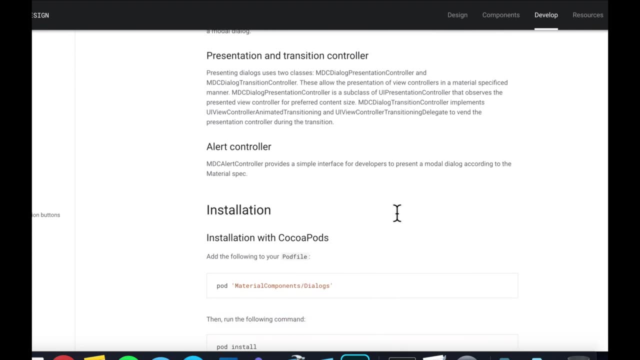 bring in each of these components as a one-off instead of bringing in the entire library. and the reason is is the library, of course, is very large and it increases your app size. so if you scroll down and you find the installation, you'll see the coco pod is material. 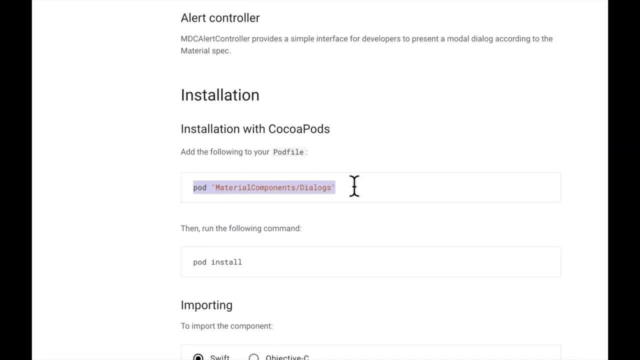 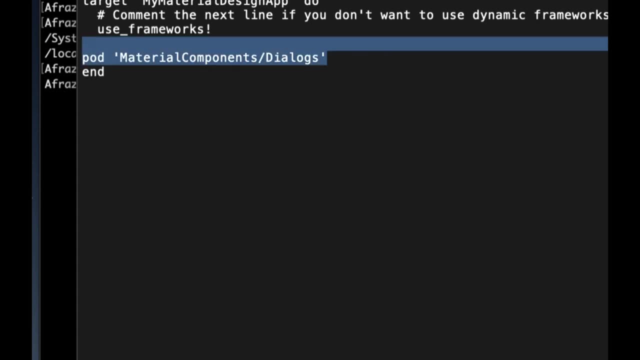 design components and then slash the thing you're bringing in. so we're going to copy that pod and we're going to paste it right here and we'll copy and paste it again. and the other one we're going to want to bring in is action sheets, and i think it's capitalized like that. let's double. 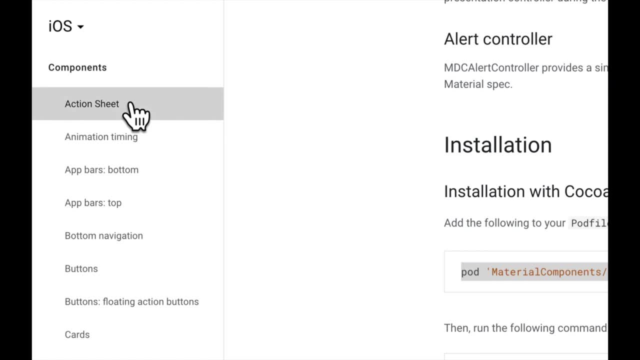 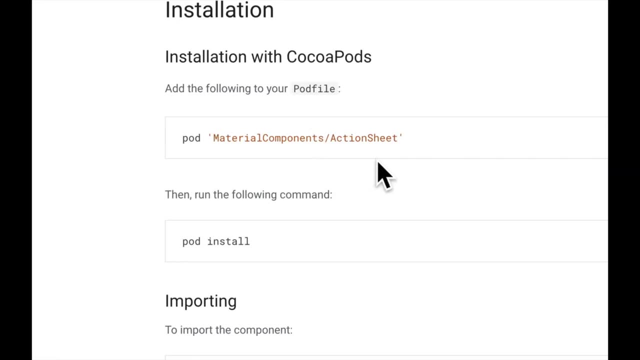 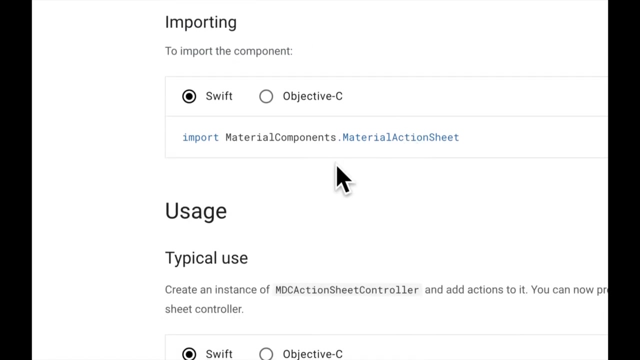 check. so let's come on over here and click on action sheets, scroll down past all the documentation that people love to not read, and we have action sheets- singular- and what's cool is, uh, it actually even tells you like how to ins, like implement all of this stuff- documentation. 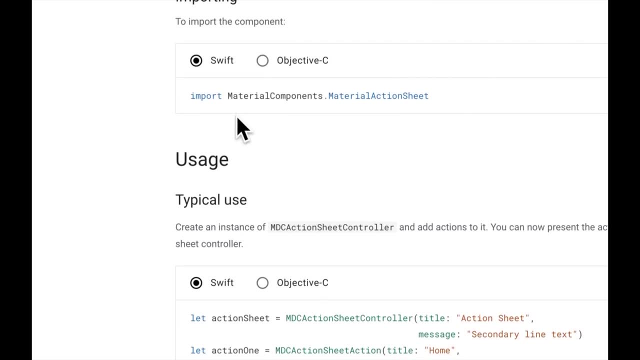 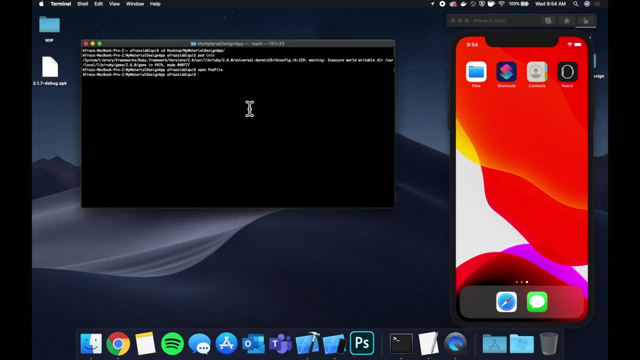 aside, it gives you basically all the code you need, so we're going to actually copy it straight up from here. so i'm going to copy the import statement that we're going to use in a second. so close up a text editor over here and run pod install- and i've actually personally used both. 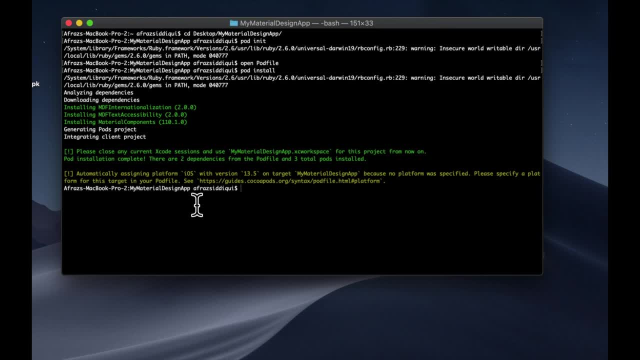 of these components in a lot of my own apps and they look really nice, they're really clean and they give you a little bit of a differentiating factor from the typical system alerts. now, i mean, design is very subjective, but i think it's interesting to see that this is available to. 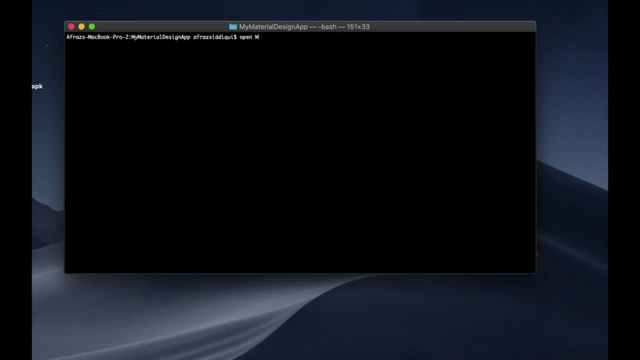 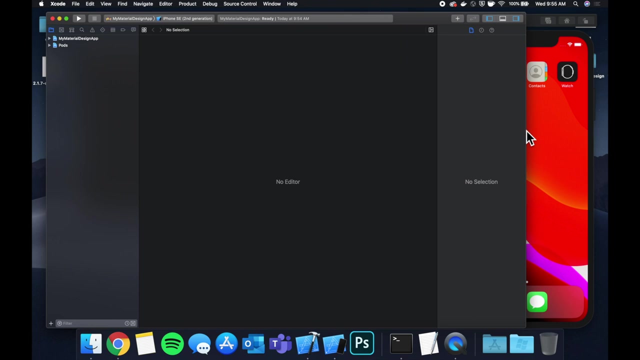 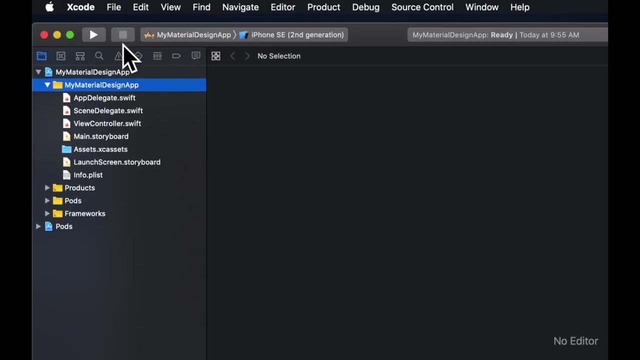 you all. so now that it has installed, we can run it, and we're going to go ahead and install it and run open the project namexc workspace and let's go ahead and expand our xcode window to give ourselves a little more room to work. let's open up this project and let me select the 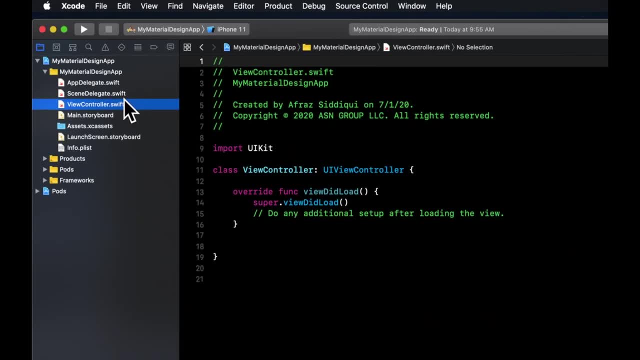 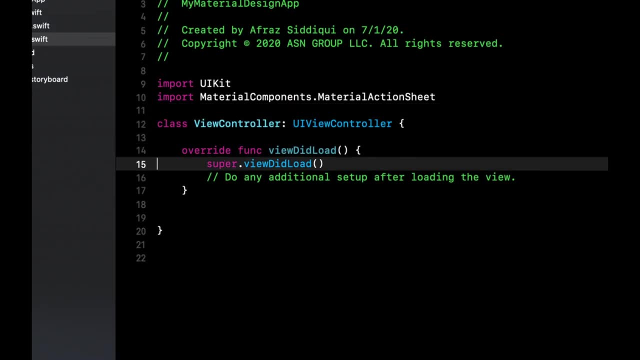 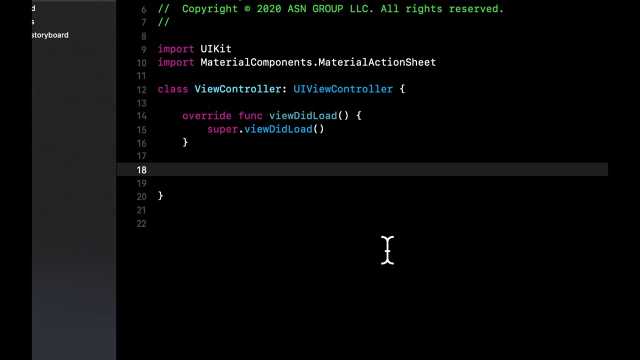 simulator. so we've got the 11 open, so we're going to stick with that. let's paste in that import and before we actually hit run, try to compile. make sure it works. after installation. let's go ahead and just add two buttons to our screen. the first one, we're going to show the dialog, aka alert, and the second one will show the action. 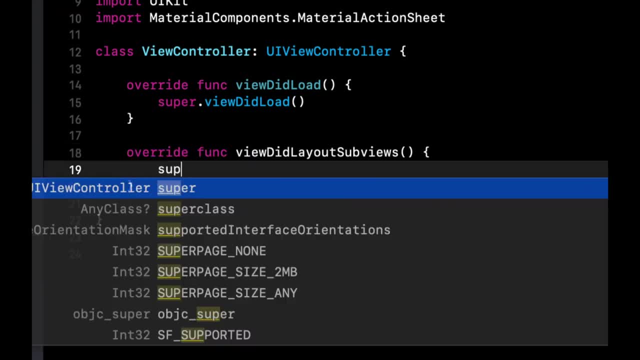 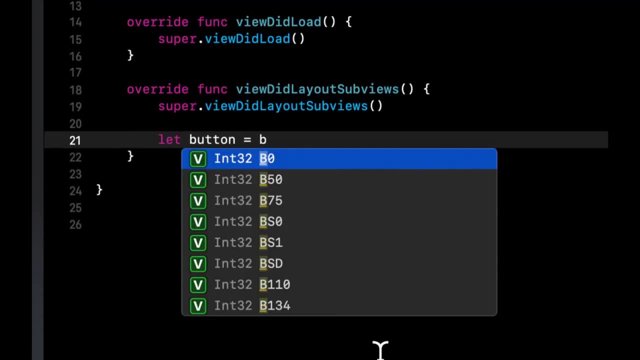 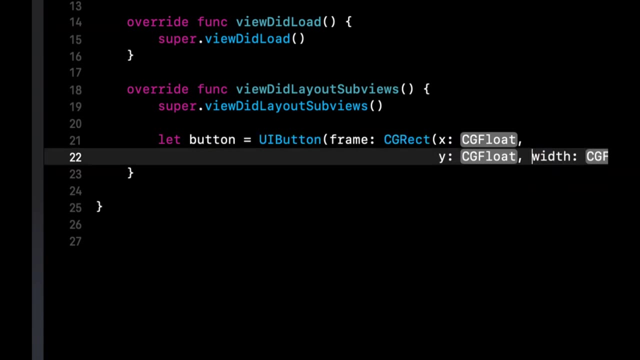 sheet. so go ahead and override view. did layout sub views? call super for that function and we're going to show a button. so the first button is simply going to be standard ui button, the c, direct, x, y, width and height. so let's go ahead and put these on new lines. this will be 220, 50. 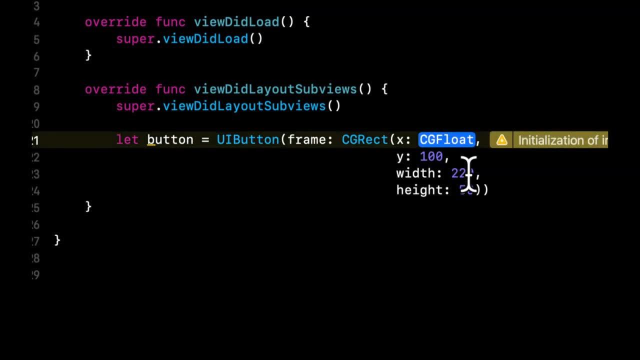 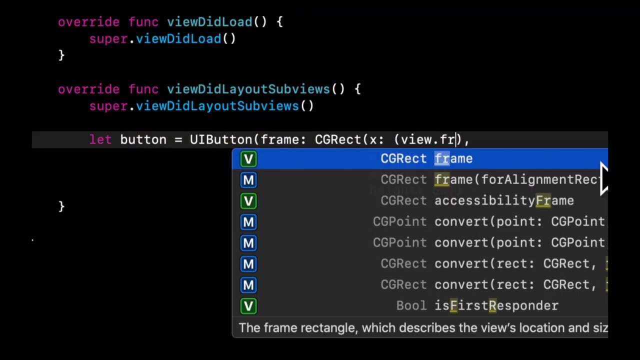 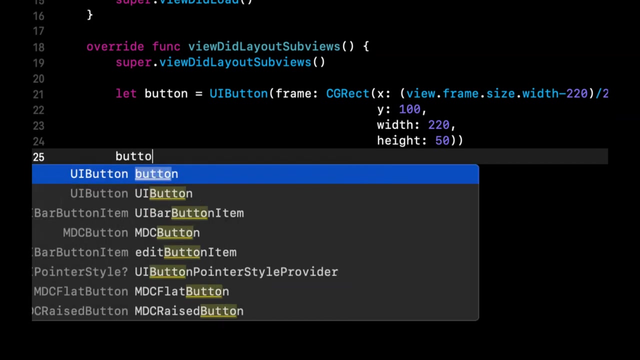 100 and we're going to make this centered horizontally. so let's copy the width and we're going to say this is view dot frame size width minus the button width divided by two. let's also give this a title and this is going to be alert for normal. 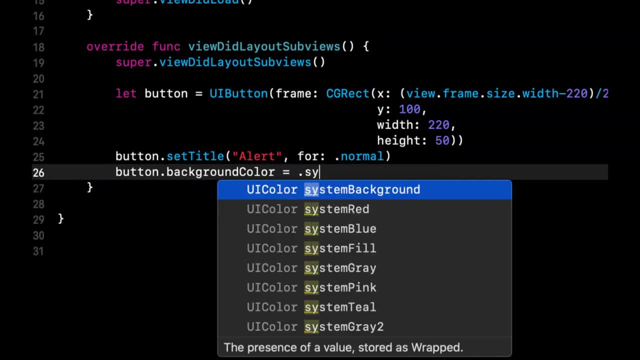 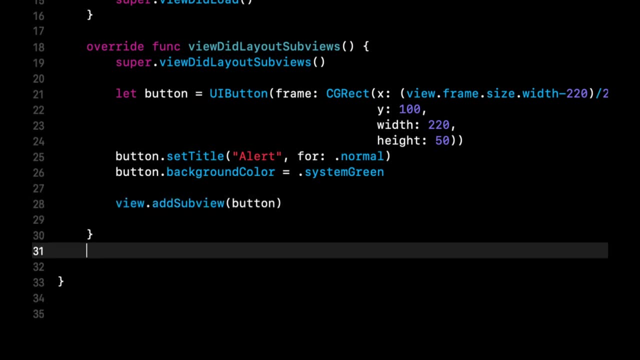 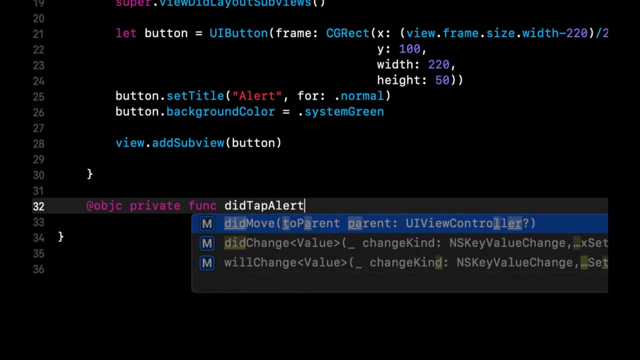 let's also give it a background color, let's go with system green, let's add it to our screen. and then, most importantly, we also want two functions that will get triggered when we tap on each button. so first one's going to be did- tap alert- and the next one is going to be 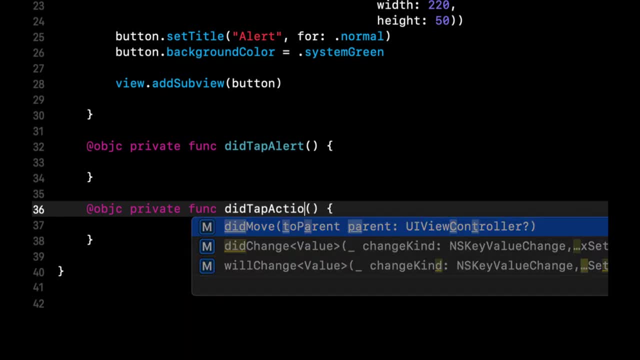 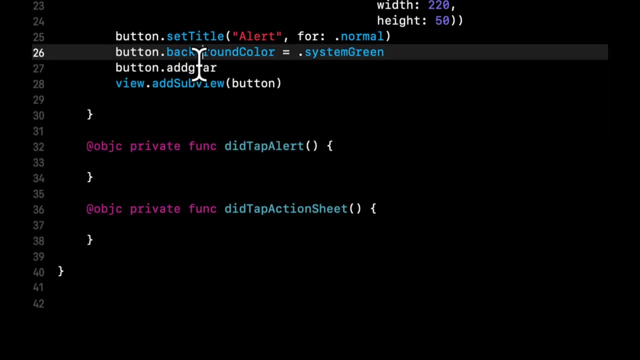 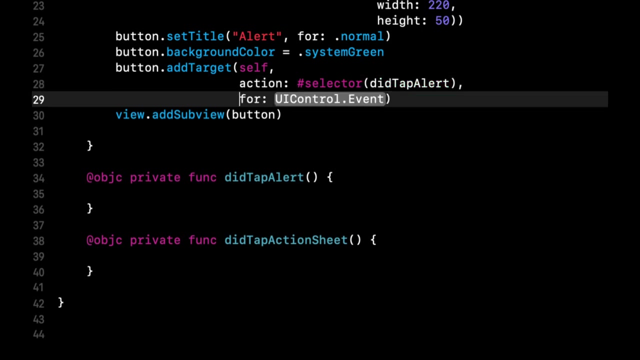 did tap action sheet. let's go ahead and add those targets. so the first button is going to be add target self action is did tap alert and this is going to be touch up inside. now we can be lazy and copy and paste this button right below it. 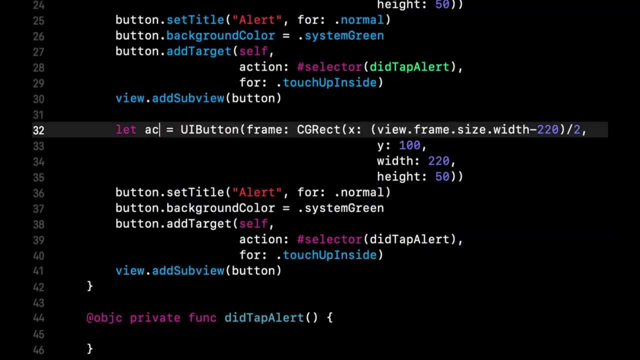 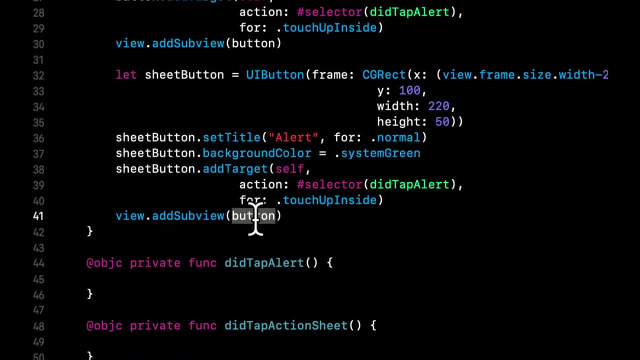 go ahead and highlight and hit ctrl i to fix that indentation and let's change the button name to sheet button. change up all of these, change this to be system blue and this is going to be a. there we go. so we go ahead and tap action sheet. let's do for this 200, so the buttons don't. 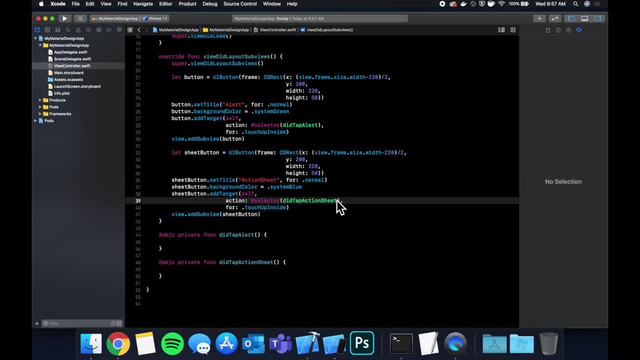 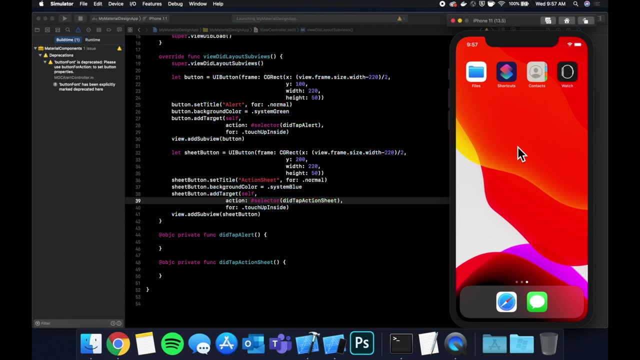 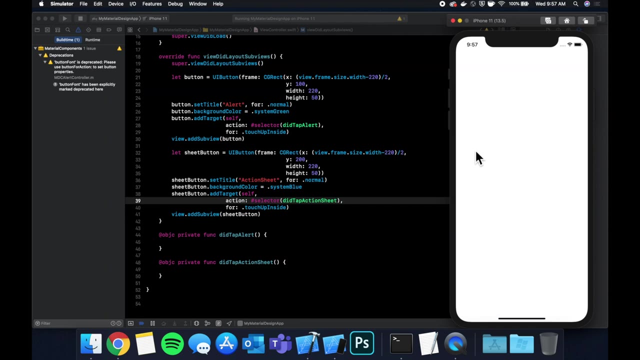 overlap and did tap action sheets. so go ahead and hit command r to build and run, and we should have our app compiling and our two buttons showing up here and there it goes. and do we have our buttons? give it a second while it decides to be slow there. they are okay, cool. so we've got a green button and 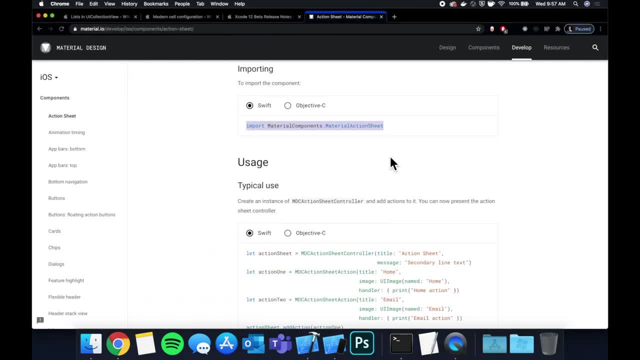 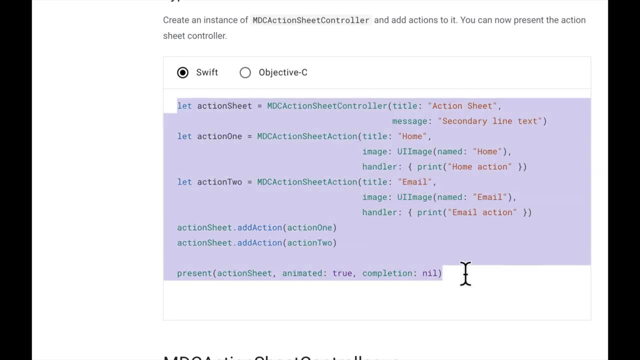 our blue button right now. obviously, they don't do anything. one that we had open here, i think, was the action sheet, so it shows you usage and you can actually literally copy and paste this. this shows you how to set it up in a basic way, and there's a lot of. 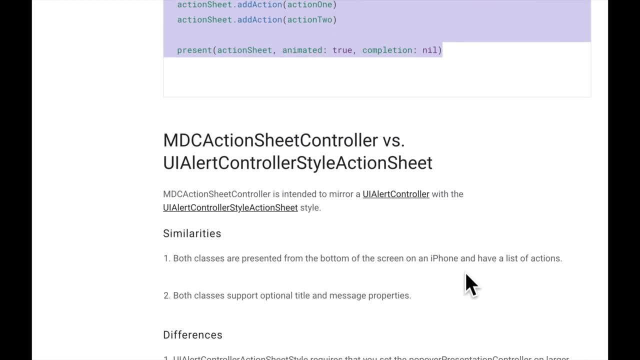 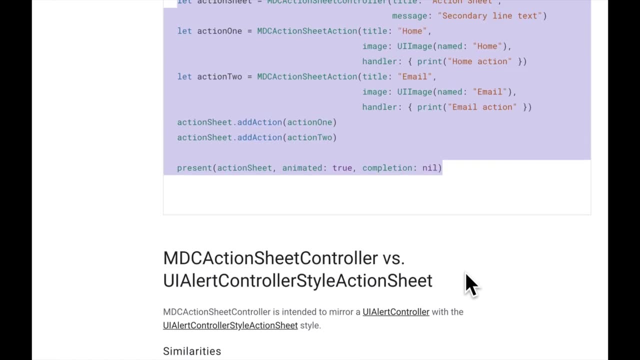 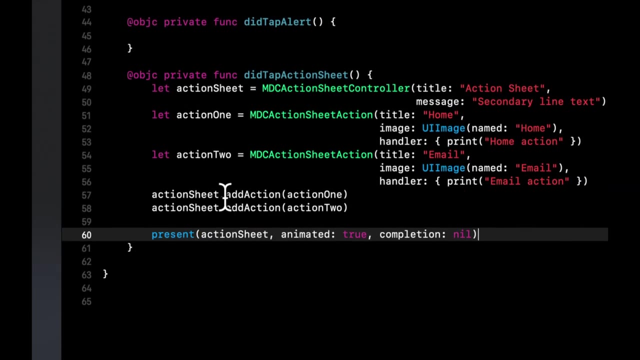 customization you can do and it kind of tells you the different styles it has, how to support accessibility, customization, all that good stuff. but i'll let you guys read that on your own time to customize it to your own desire. but for the action sheet we're gonna paste that stuff in here. 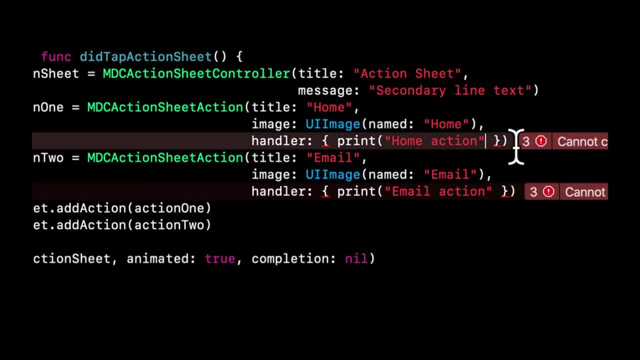 and google actually, surprisingly, has a typo in this. they forgot the parenthesis for the closing of the print, and they also forgot the parameter that comes in, so do the underscore in. since we don't care about the parameter, i'm also going to line break this on a new line. 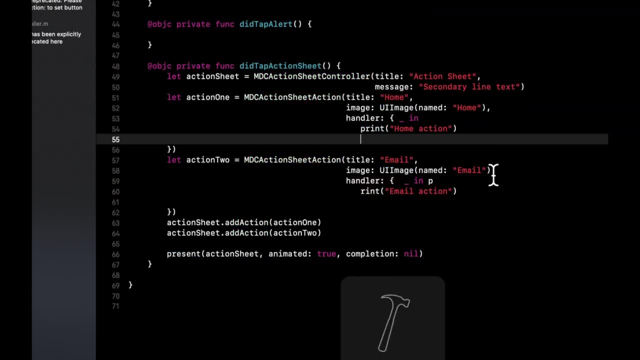 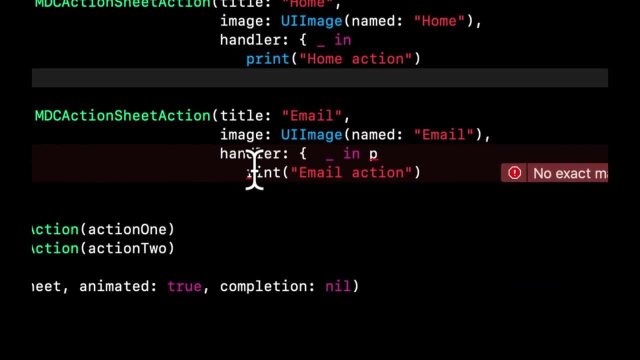 like that. and actually, if you just say command b, this should be good to go. looks like we have an error somewhere in here, so let's find it. so let's see we have. oh, it's because i put the line break after the p, so go ahead and hit command. 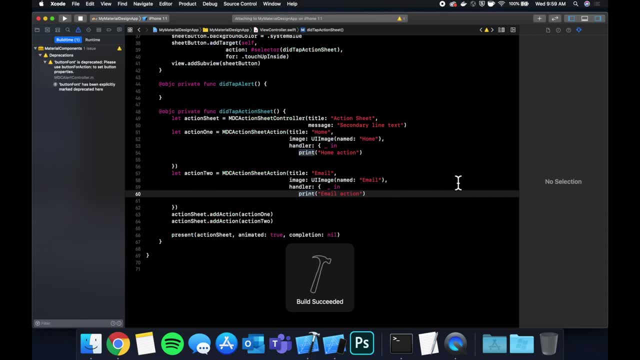 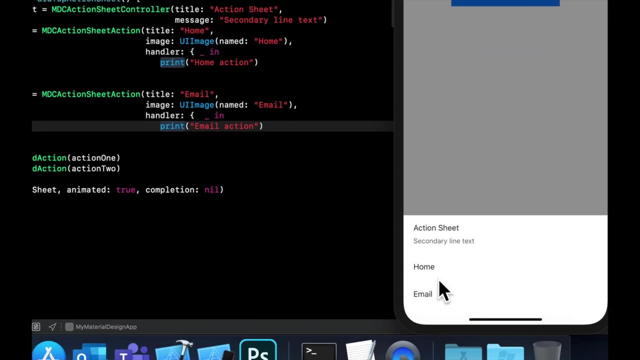 v now and their code for the most part is uh functional, but we're going to look at some customization. so if you go ahead and hit this, you'll get the action sheet showing up. you'll see no images actually show up because it's trying to use images that are supposedly in. 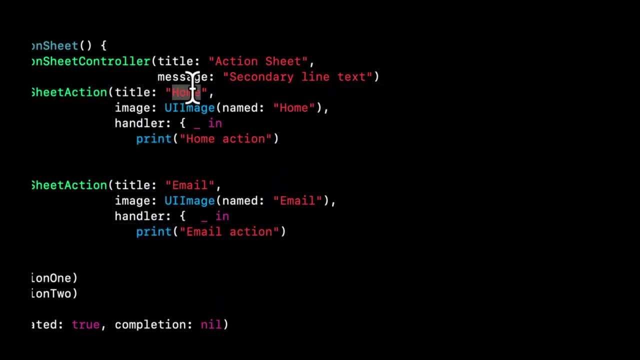 our xc assets. now those don't exist. so i'm gonna change this to be a system symbol and we're going to stick with a house, and then this one is going to be a system symbol as well for gear, and this one will be settings. so if you hit command r again, you'll see that we now should have. 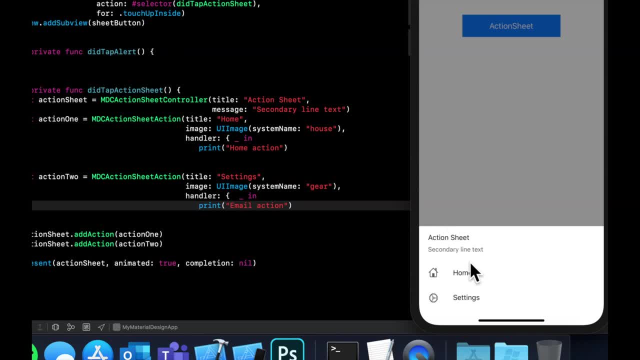 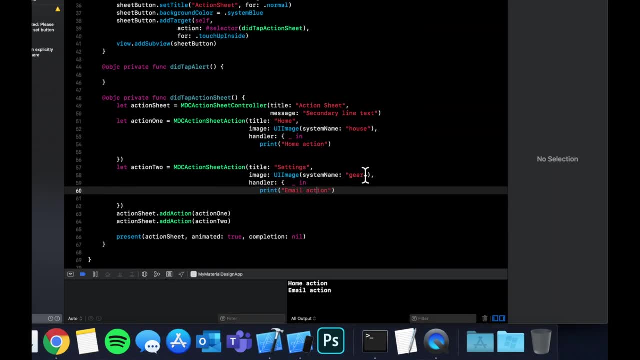 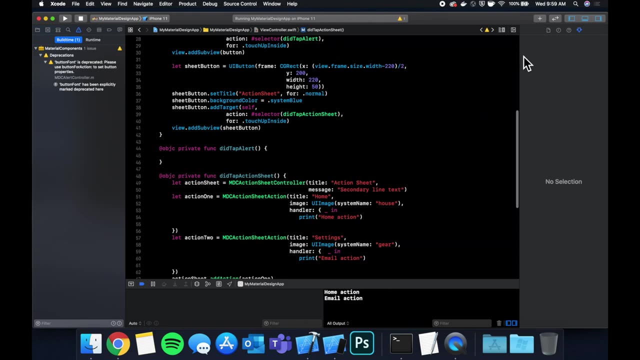 our icons. we've got a title or label as well as our buttons in the actual sheet and we tap on them we get the respective print statement out. so pretty simple to set this guy up. so we'll look at a little basic customization in a second after we bring in the alert and close up that. 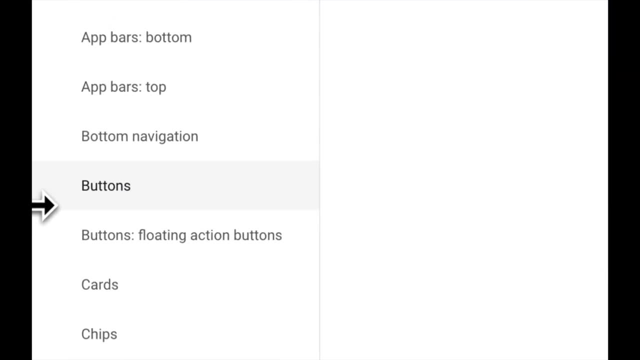 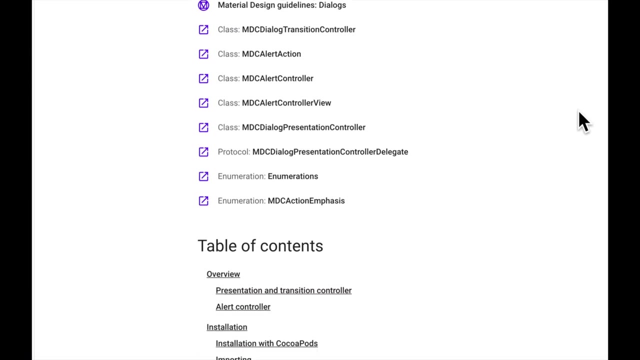 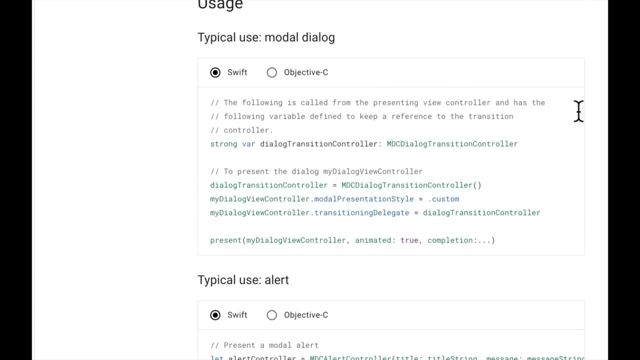 so we're going to go to the console and let's go find the alert documentation- uh, that they call a dialogue. so we're going to go to dialogues and let's see, let's come down here and try to find what we need. so we're going to want an import and i think i already know the import is. so i will. 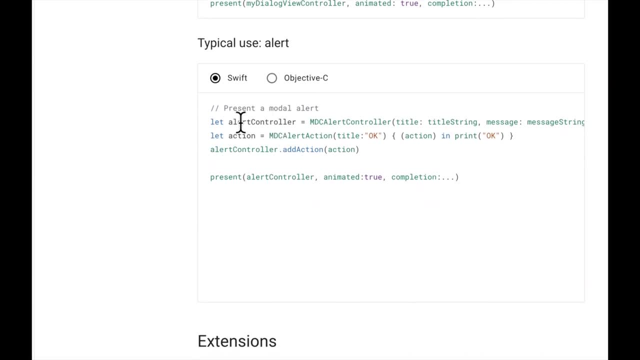 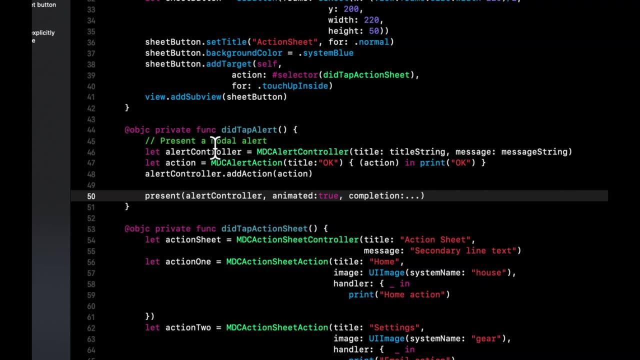 skip that and let's see typically user alert. this is what we want, so we can drag or the copy all of this jazz. come on over here and paste it in here. see, do they have any issues in their code? here looks like you need to fix this completion. 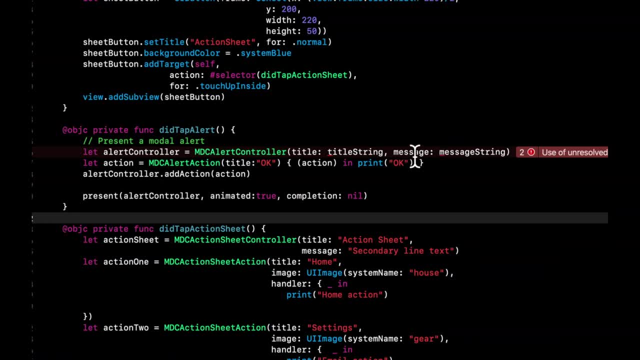 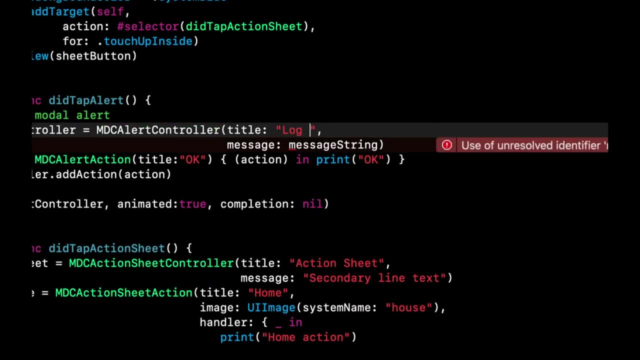 that can be nil and we got to pass in a title and a message. so let's say you have an alert of. let's say there's a logout alert. so let's see, log out. are you sure you would like to log out? and we are going to do. 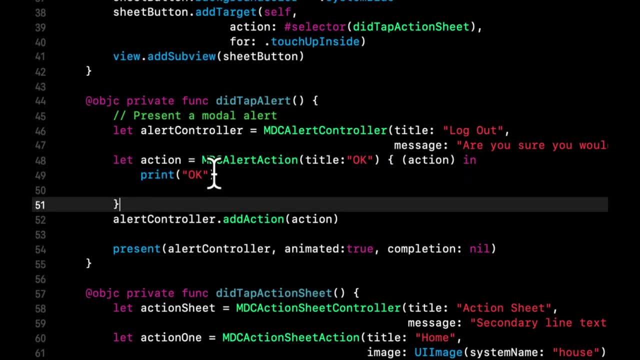 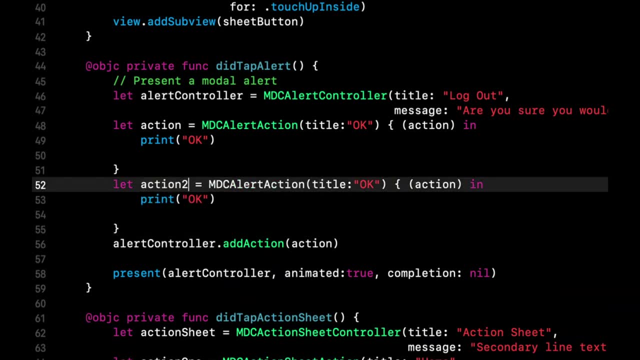 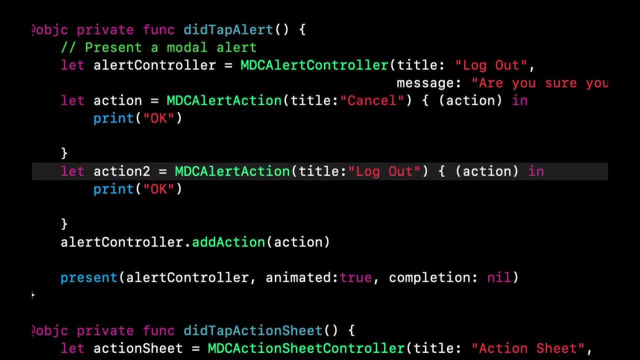 two buttons on here, so right now we just have this one and instead of assigning it to actually no, we can do it like this: so instead of uh having the one, we want two. this one is going to be cancel log out, and i think we can also specify. 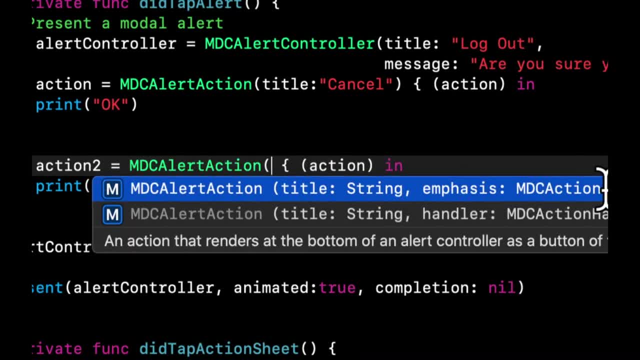 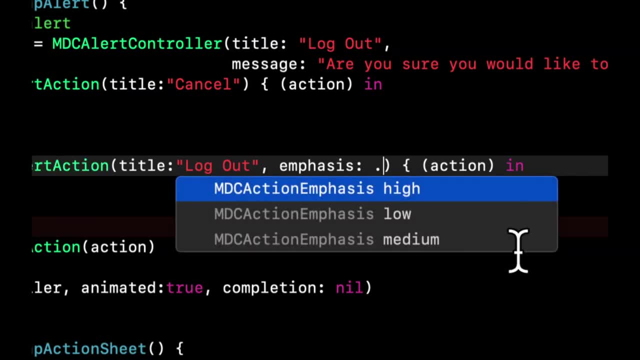 a type on here. so if we close this and reopen the constructor, uh, there's title, oh, emphasis, that's what they call it. so if we put in another parameter in here for emphasis, there's a couple types: there's low, medium and high, and it controls the bolding or how bold, rather. 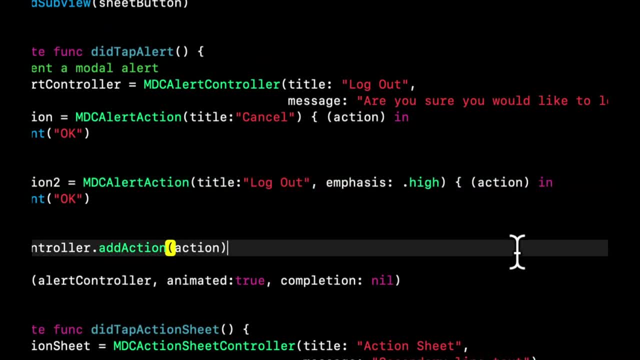 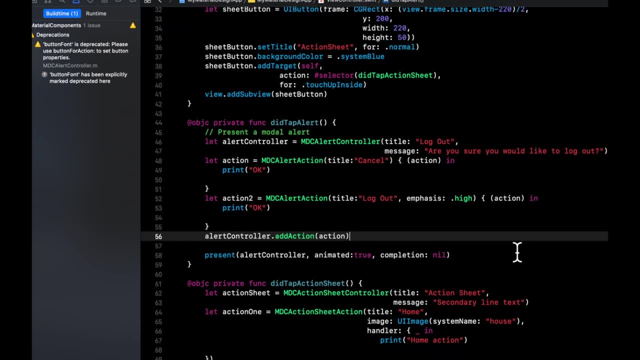 the thing shows up as, so I'll make this one that so. it should be slightly more bold, and I think that's all we really need. so go ahead and hit command R. we have that warning because we're not using the action, and let's go ahead and 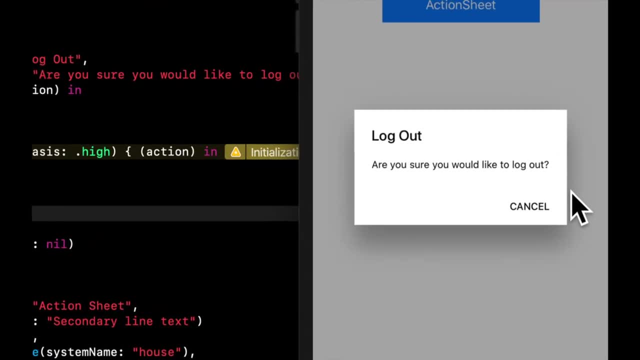 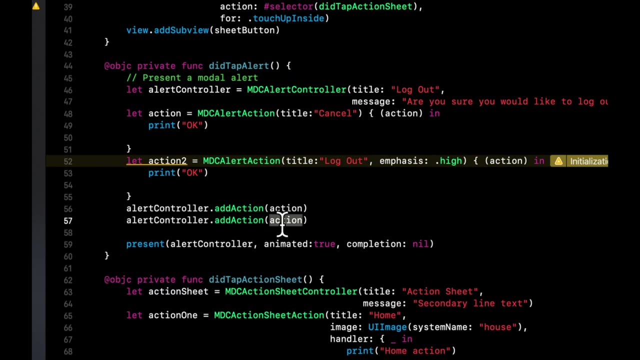 hit this button and you'll see our super nifty looking alert here. so we have cancel. well, where's the other one? right, we need to actually add the action. so let's do that. and this is action. to let me make this one action one. so we have. 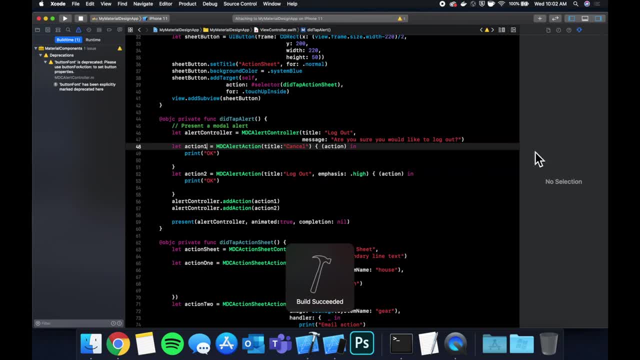 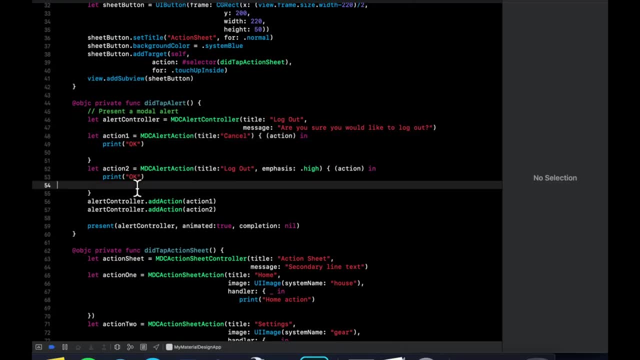 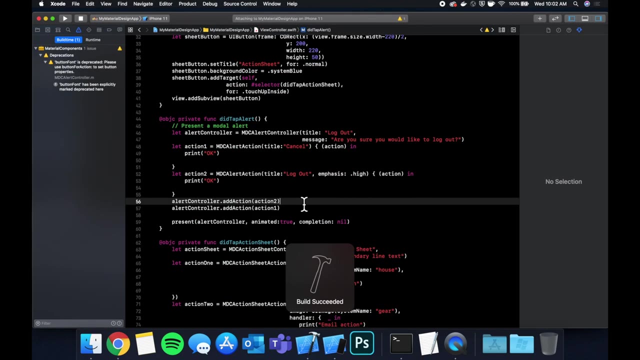 some parity. go ahead and hit command R, and I believe the order should be correct, since we added cancel first and delete second or log out. looks like I'm mistaken. it goes right to left. whoops, let's actually add this one first and then action one, and logout will be. 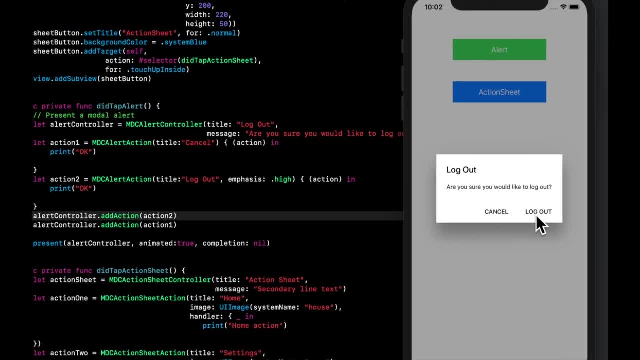 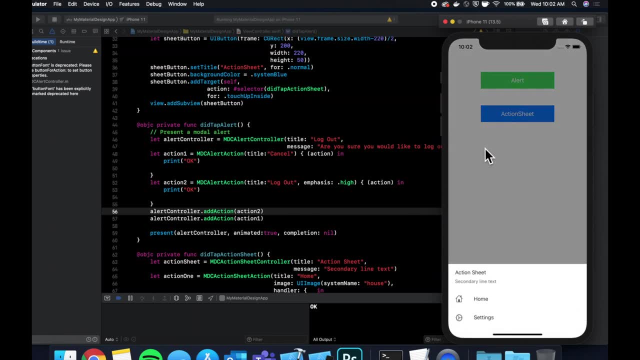 all right now we've actually created one and, like I said before, we need to on the right, like so, and whenever we tap any of these, of course we come into the closure and we get our print statement. so that's how you can do an action sheet and an alert and what's pretty. 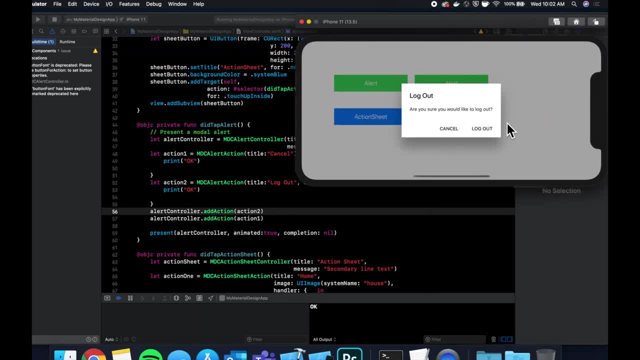 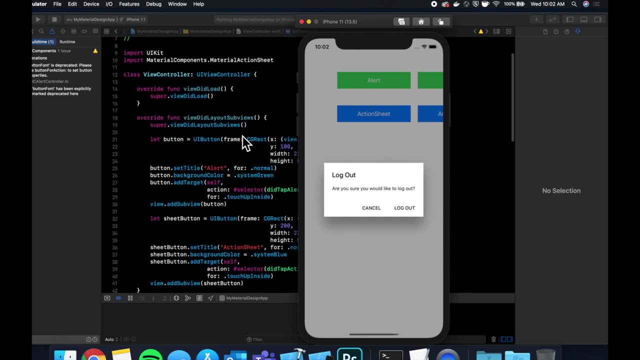 cool is like you get a bunch of customization. things like landscape and all that jazz works, but don't mind the double buttons because I put all this code in muted layout. but what we're going to look at real fast for some basic customization that most people would like to do is dark mode. 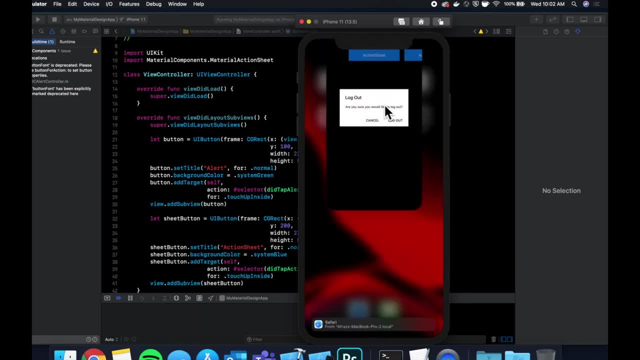 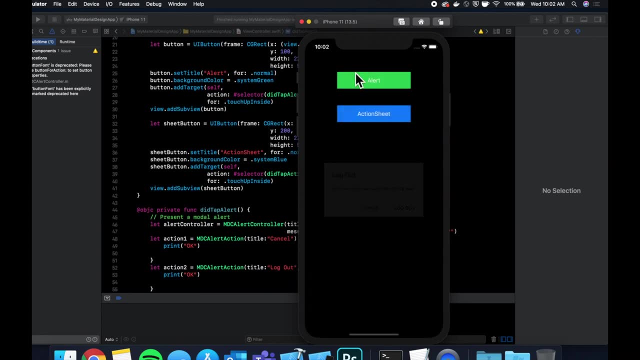 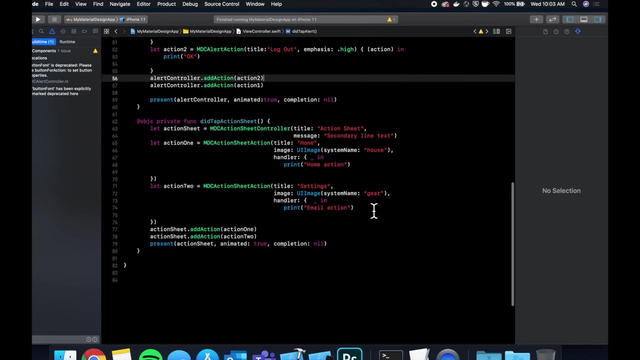 so you'll notice out of the box, if we tap on this, it's actually white and it's not dark when supportive. so like what gives and same thing for the alert. so what you can actually do- and you can definitely read the docs and figure this out, but I'll just illustrate it here- is you can specify. 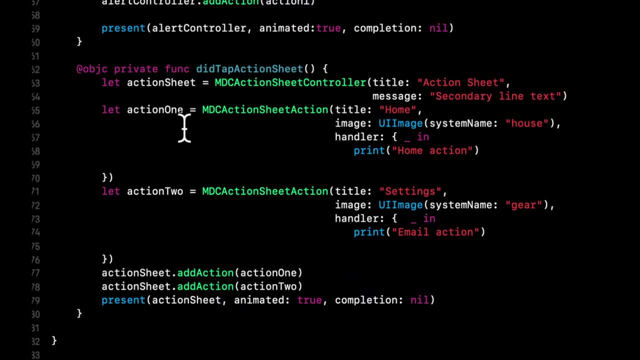 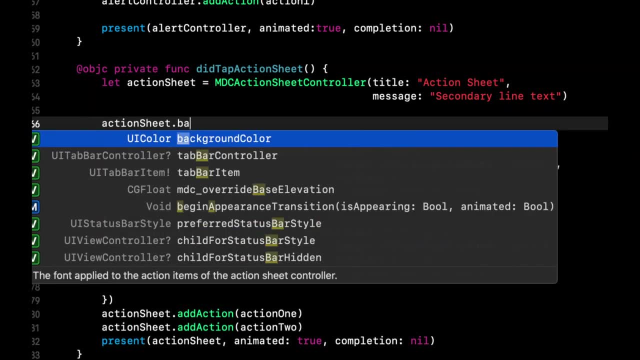 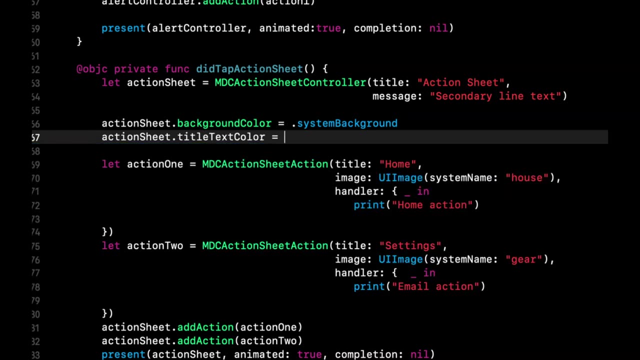 all the colors for all this stuff and like the corner radius, and you can customize basically every little nitty-gritty detail about this. so we're going to say the background color for the action sheet is system background. we're going to say the title text color is label. we're going to say the message. 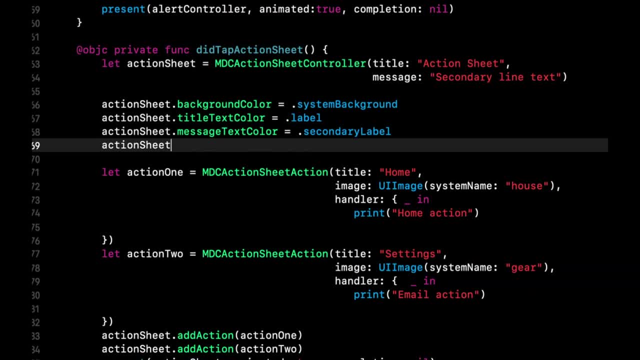 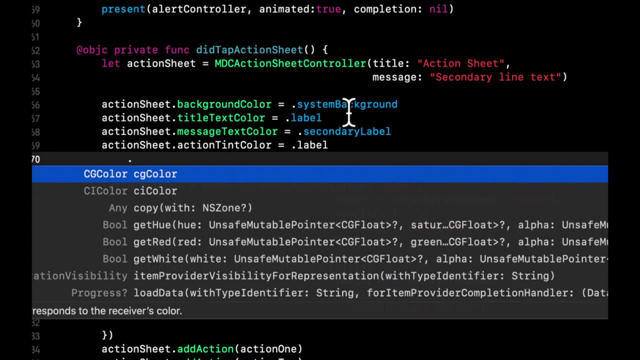 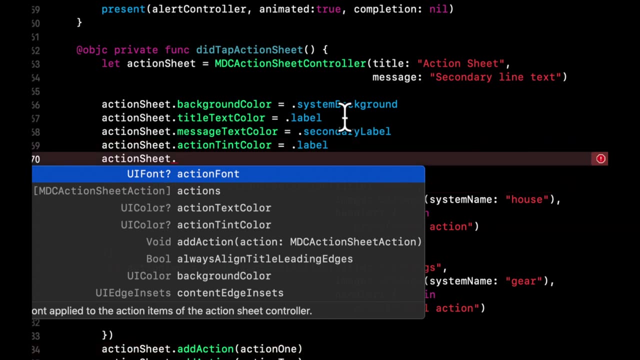 text color is secondary label and we're going to say there's a tint color on here as well- is label and these label and system label things. these are all semantic colors, if you're not familiar. so they are adapted to both dark mode and light mode. so that's that action, tint color, and I think 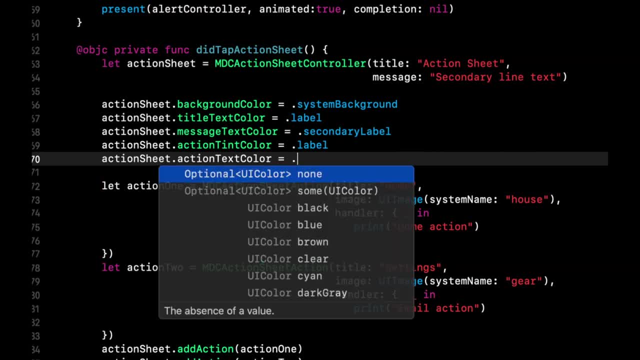 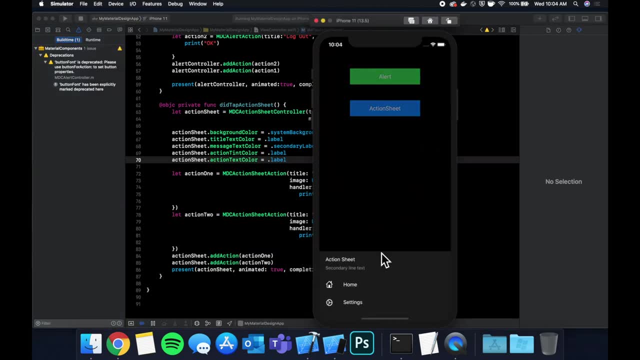 there's an action text color too, and that will also be label. so go ahead and hit Command R to build and run. let's hit this, and now our action sheet looks a lot like what YouTube's action sheet looks like. we've got the system themed background. 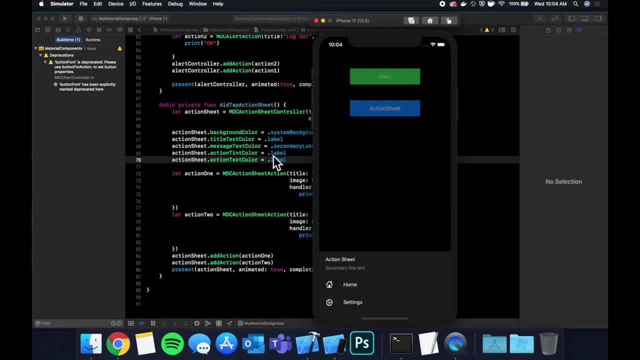 title: color stories: action background- accessibleSU 활동. Subtitle is like a little bit lighter because it's secondary. We've made it and then we have white for the icons and the Action label text. so now you can- you can assign any color you want, is the point, but dark mode. 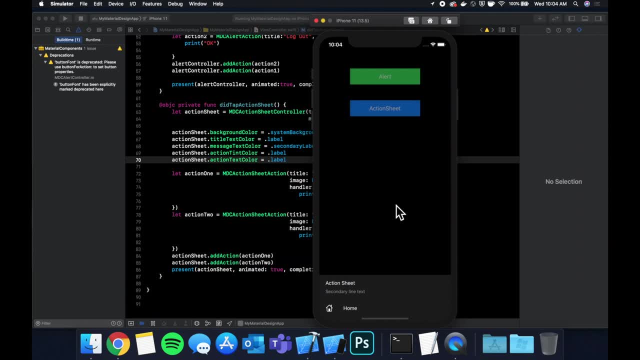 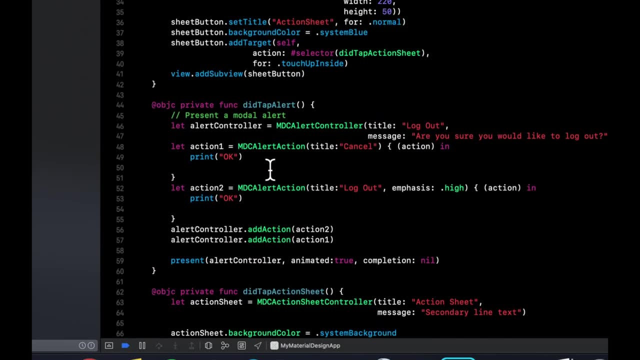 Obviously people like to support and it's pretty expected by users these days. So it's definitely important that it doesn't look obnoxious like this, So you can actually apply all of this stuff on the alert as well. So let's see if memory serves and I can do it. 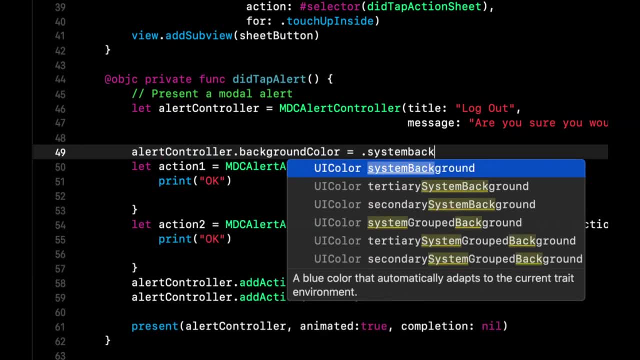 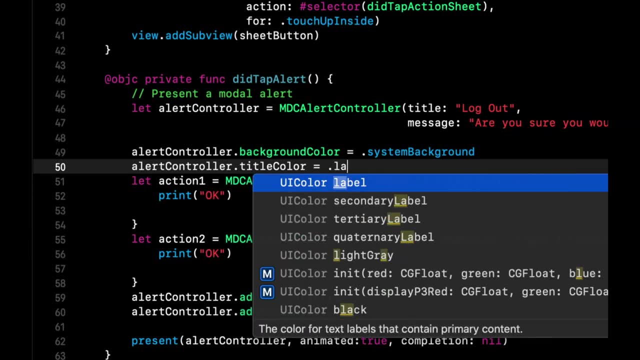 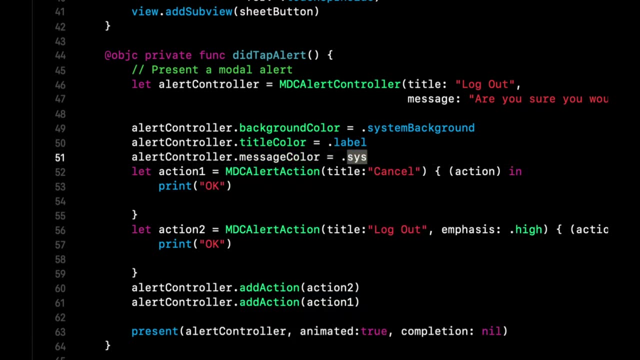 I think the properties are pretty similar actually. So you're gonna have a title text color, Title color rather, And let's see, I think there's a message color. This one should be secondary label. Well, it doesn't have to be secondary label, but I'm gonna make a secondary label and 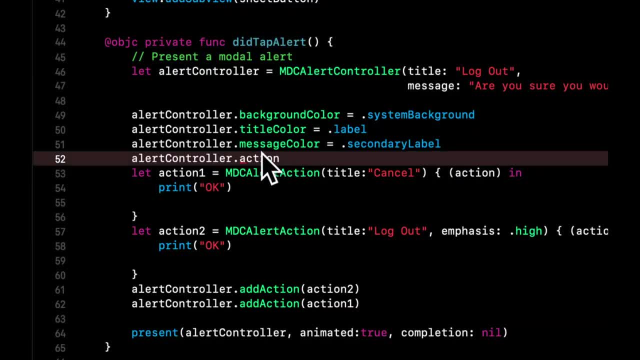 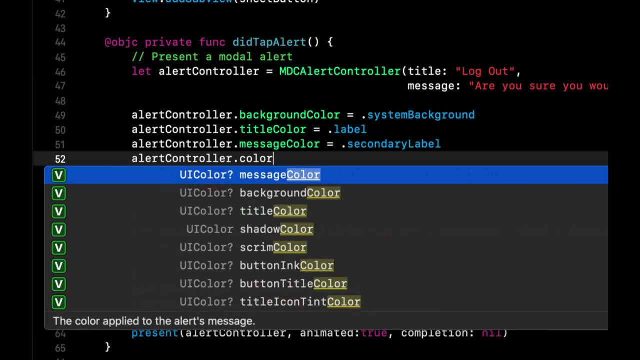 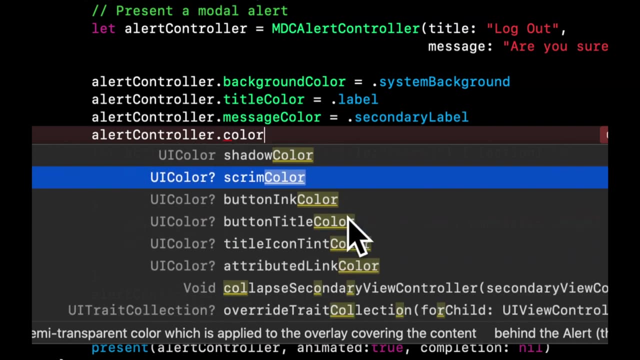 I think this should be an action color. It's closed me antivirus pop-up. Let's see there's action. Should be another color on here. Let's see this title color, the shadow color. There's Scrim color, message color, background color, Button ink color. I think we want button title color. 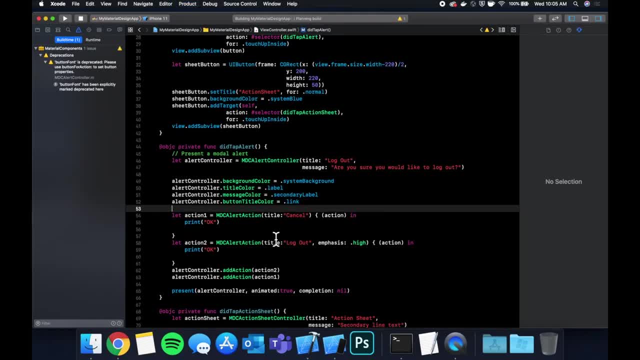 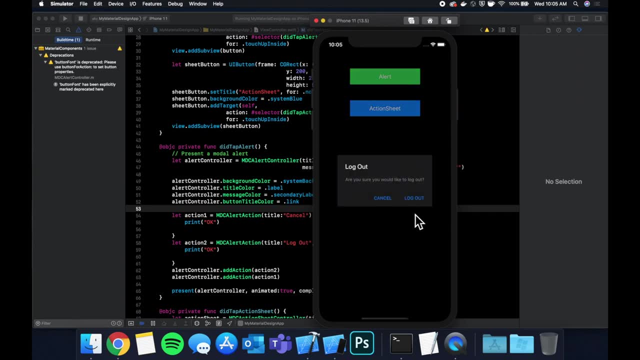 And I actually like this being like blue. it makes it pop a little bit more, So you can leave it the standard or make it link. now we hit this, we'll get this, and this is exactly, almost verbatim, What Google is pop-ups look like and 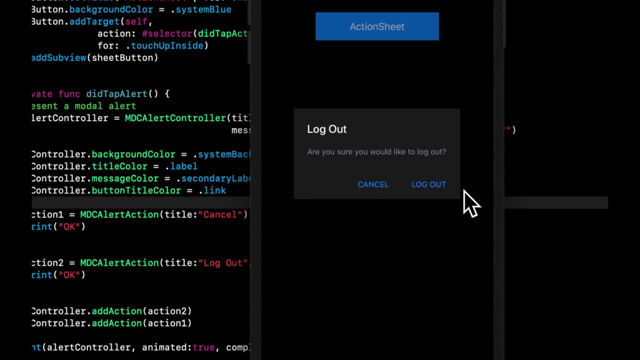 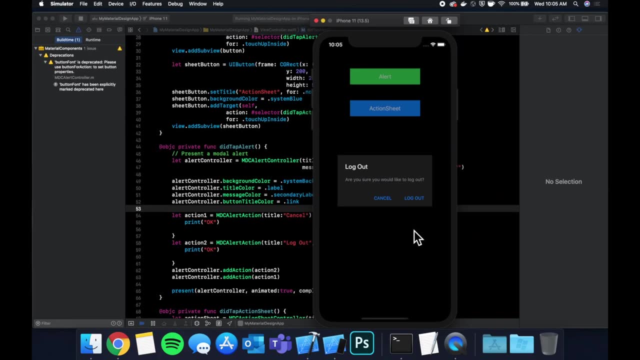 Let's say you wanted to log out to be read. you can do that as well. just to indicate that it's, I guess, a destructive action, as Apple calls it, something that the user should just be careful about tapping. and Let's actually run this on iPad and see what it looks like on iPad as well. 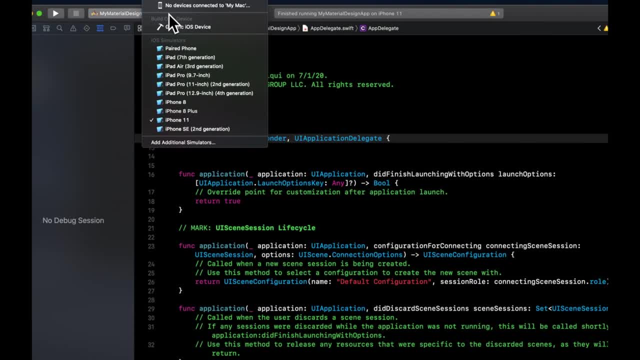 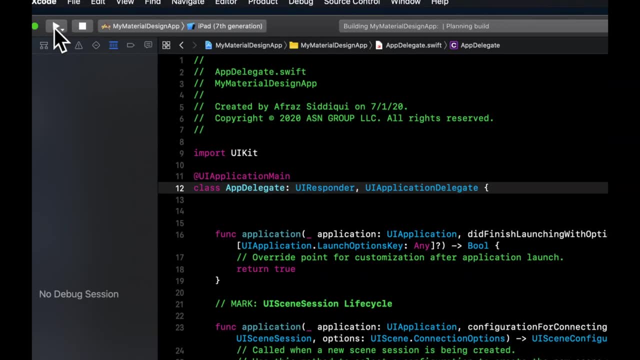 So I'm gonna close that app crash, obviously because we closed the simulator. So let's go ahead and let's pick the iPad 7th gen. Go ahead and hit, run over there And just to show you guys what things look like. so the action sheet on iPad. 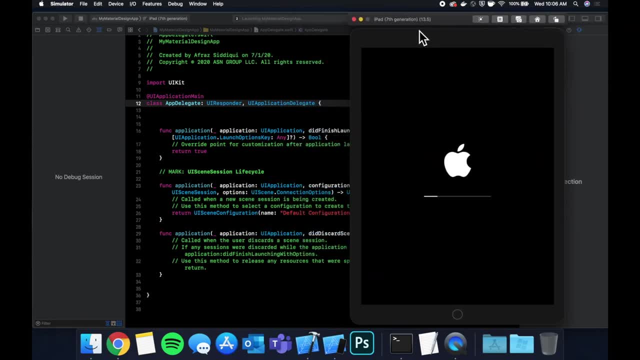 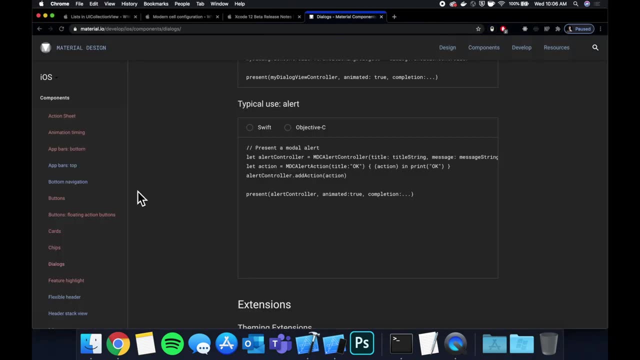 looks a little interesting if Our simulator decides to not be slow and load and while it's doing that, actually Let me switch this to dark mode. while it's doing that, you can come through this list and you'll realize it's pretty extensive. We got dialogues, feature highlights. 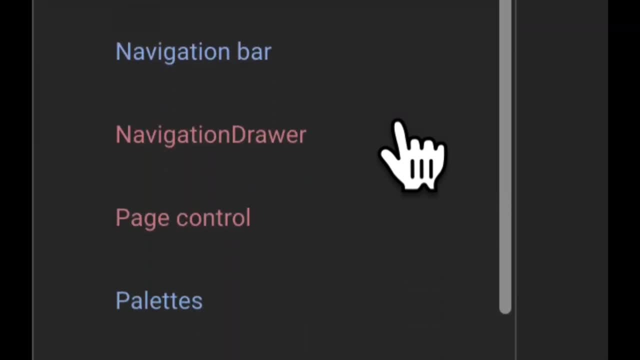 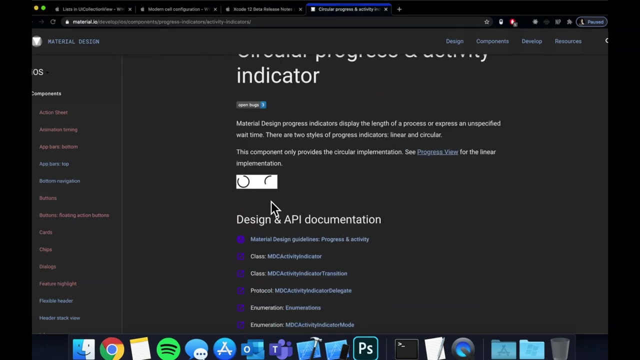 flexible headers. Library info list. there's the list kind of goes on and on. progress indicators are actually pretty nifty Ripple effects. so I actually like this circular progress indicator that they have And looks like they don't have a preview here. actually they do. so there's a. there's a bunch of other libraries. 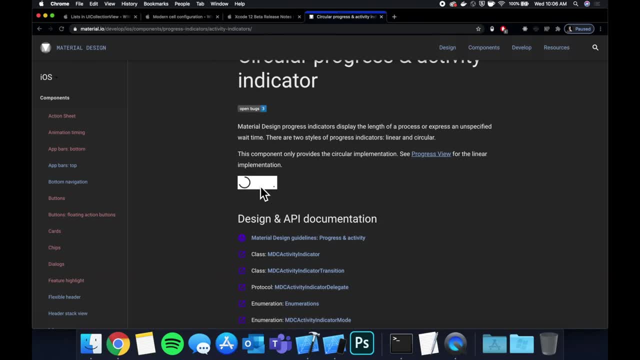 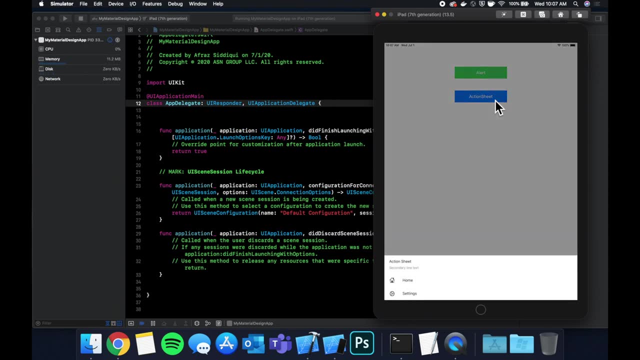 That can handle this like progress. HUD is very popular, but it's nice to be able to get all your components from Google. But now that this has booted, we can hit this and we see the action sheet is similar to how, again, Google Does it, whereas if you did it on 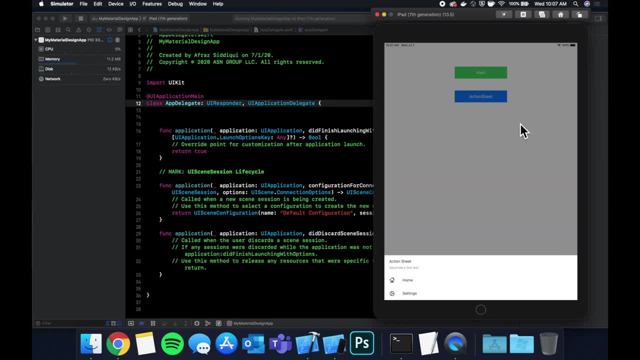 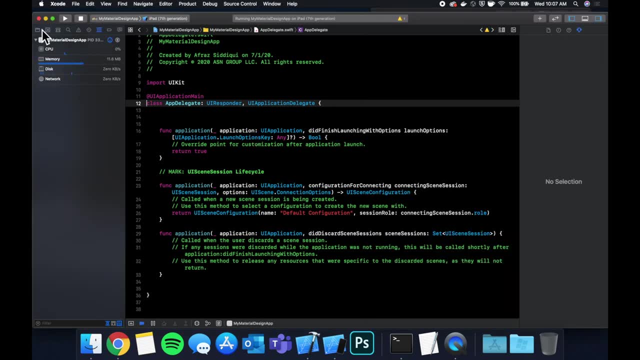 Use a normal Apple action sheet. it would be kind of a pop-up with like a pointer so you can customize everything the way you want. But this is a great resource that I figured I would share with all of you. So that is all I had. I'm gonna end this video before my fan decides to be obnoxiously loud. 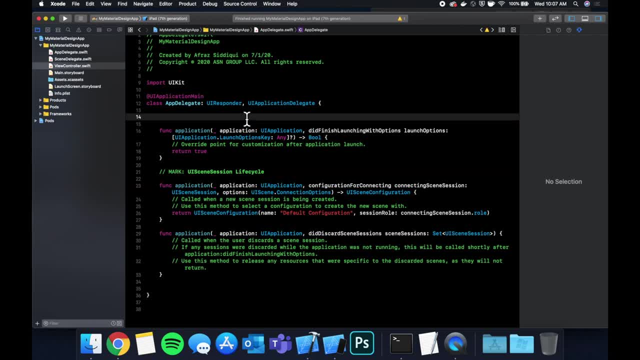 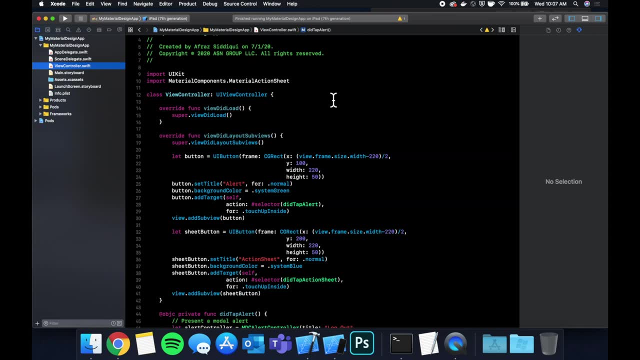 If you haven't hit that like button already, make sure to do so, for the YouTube algorithm helps out the videos quite a bit. Helps me make more content for all of you. if you're new to the channel, Hit subscribe while you're at it, if you have any comments. 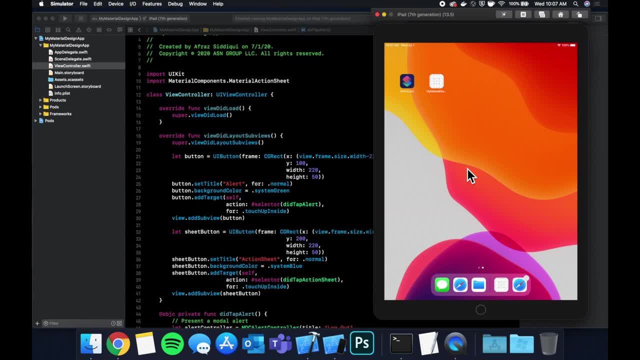 Suggestions, feedback, etc. etc. don't hesitate to leave it down below. Thanks for watching and I'll catch you in the next video.